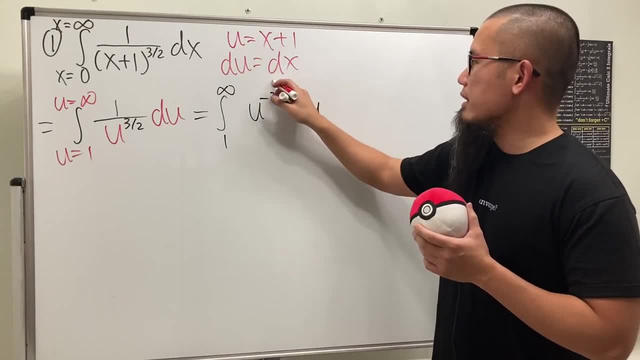 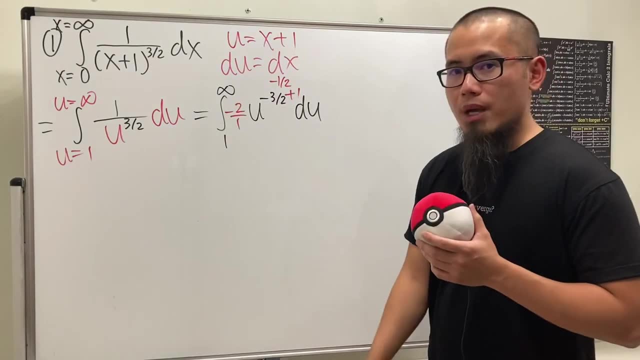 Let's integrate that. Add 1 to the power and we'll get negative 1 over 2.. And divide it by the new power. We just have to multiply by this reciprocal, namely negative 2 over 1.. So you see. 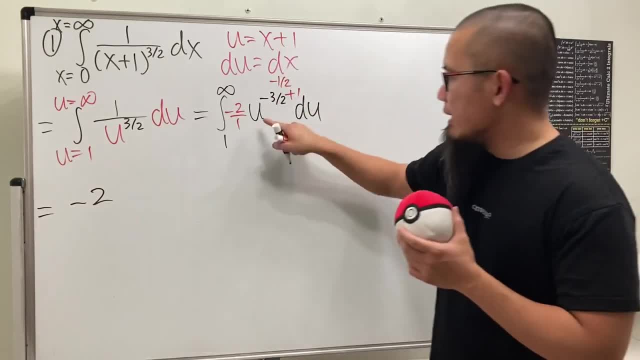 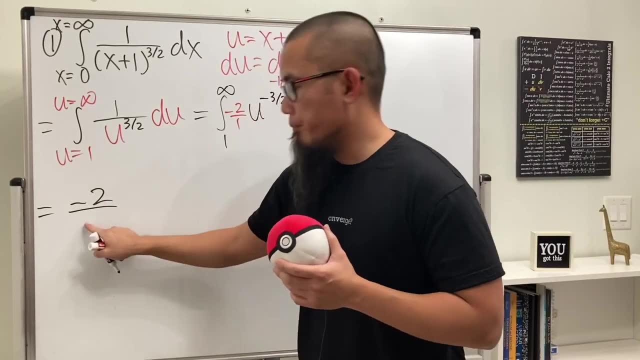 we will get negative 2, and then u to the 1 over 2 power. but that's negative. We bring that down to the denominator, So we have negative 2 over u to the 1 half, which is the same as square root. 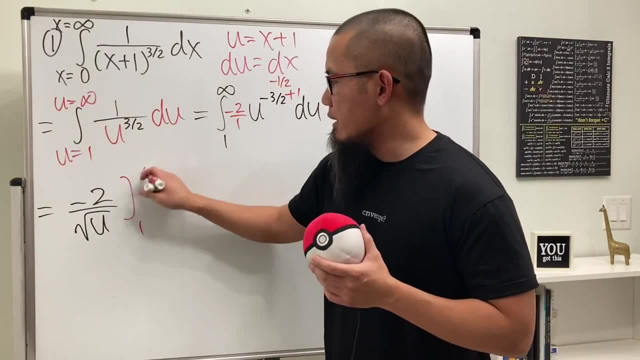 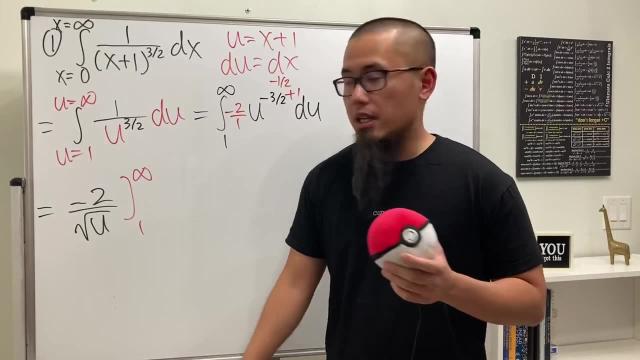 of u And right here I'm just going to be plugging 1 and also infinity. But just keep in mind, when we plug in infinity we are really taking the limit as u goes to infinity, that kind of thing. But technically you should write it as the limit as b goes to. 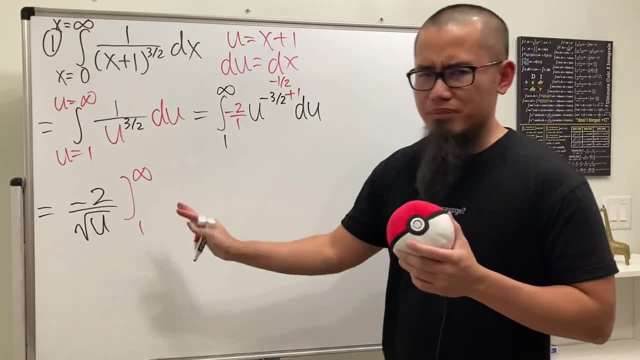 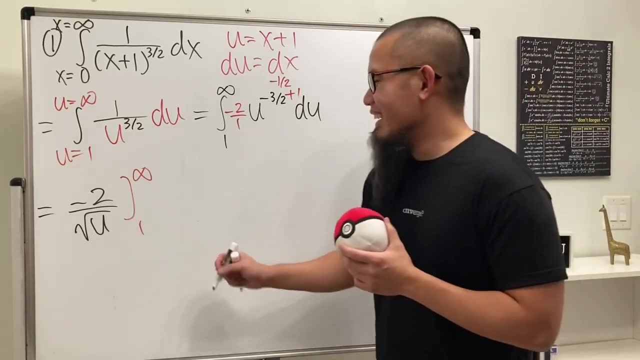 infinity, But it's easy for us to do a conclusion, so let's just do it like this: If you're taking my class, then that's okay, right, This is okay, You're good, I'm good, yeah, All right, so here. 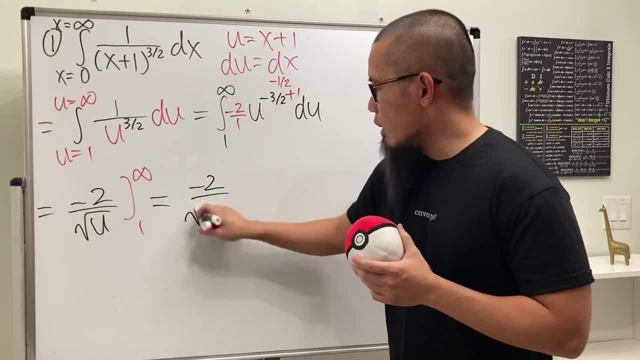 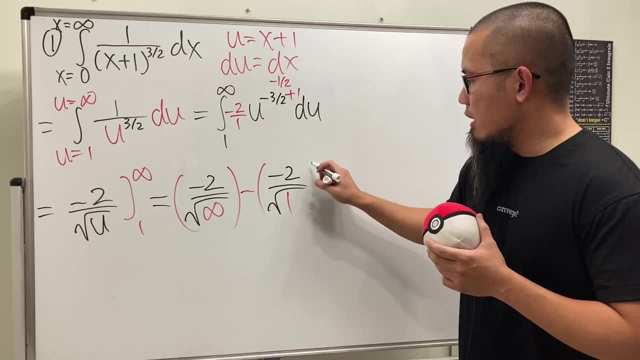 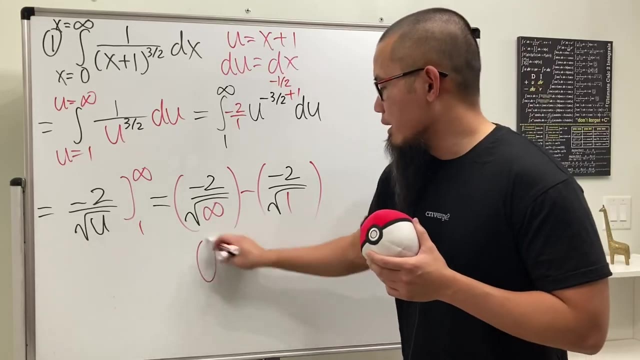 plug in, plug in and then the first term- we get negative 2 over square root of infinity, and then minus. the second term is negative 2 over square root of 1.. All right, and what's this? Negative 2 over infinity? right, So that will be 0, and then this is just going to be plus 2.. So 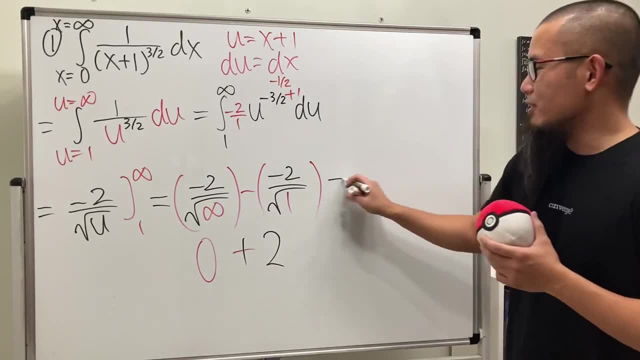 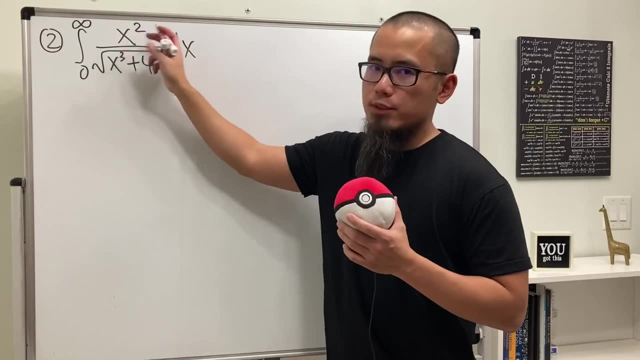 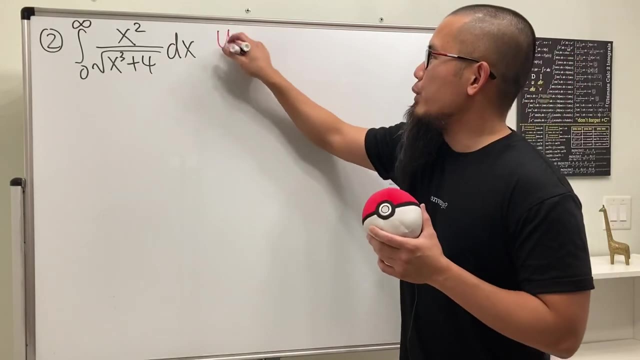 minus times a minus, and then we have the 2.. So, ladies and gentlemen, the answer for the first one is just a 2.. For the second one, we have the integral going from 0 to infinity of x squared 4.. Can we do u sub? Yes, So let's do u sub. Let u equal this x to the third power plus 4,. 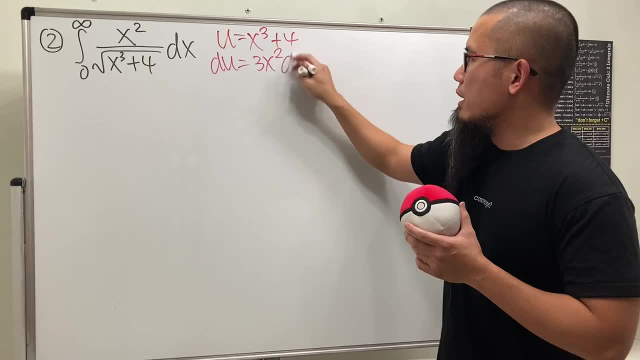 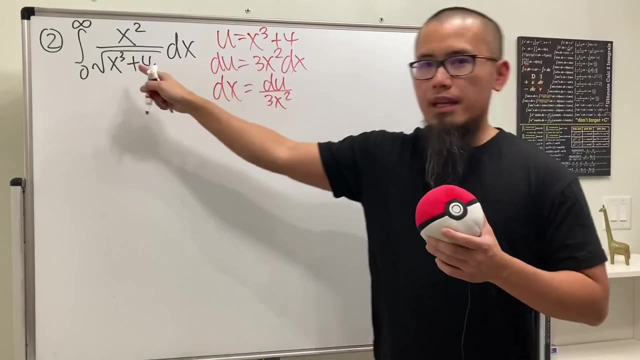 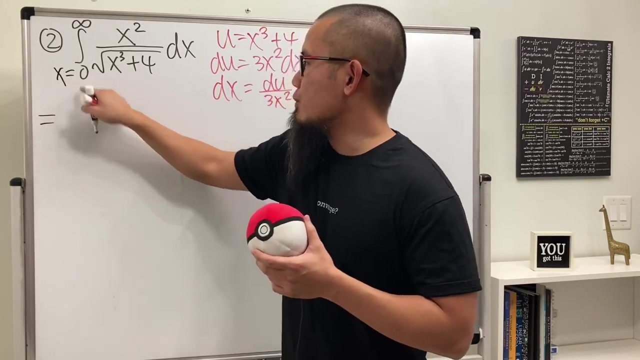 and then differentiate both sides. du is 3x squared dx. Divide this on both sides, dx is equal to du over 3x squared. Then take this integral to the? u world, the happiest place for integration, right? All right. so we see when x is going to be 0 here. put it here. 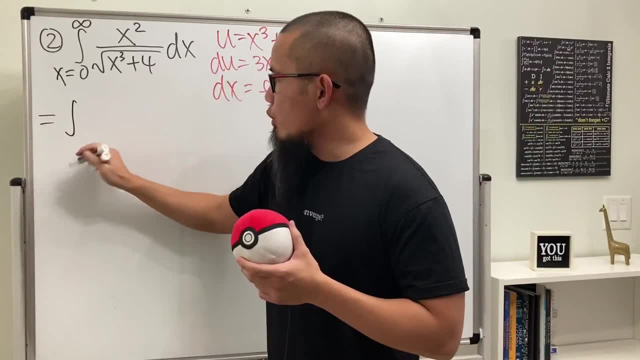 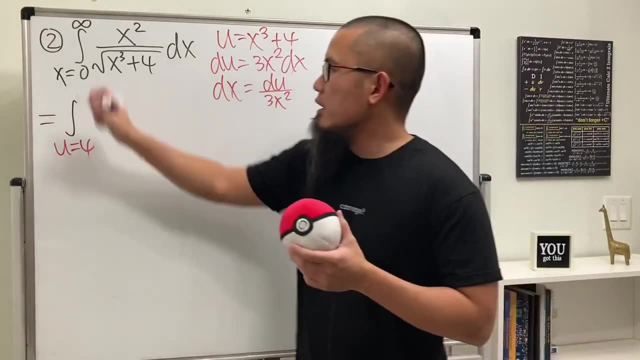 0 to the third power plus 4 is 4.. So we have integral going from 4 and put infinity to here. Infinity to the third power is infinity plus 4 is 2 infinity. So when x approaches infinity, you know u approaches infinity as well. And then here: 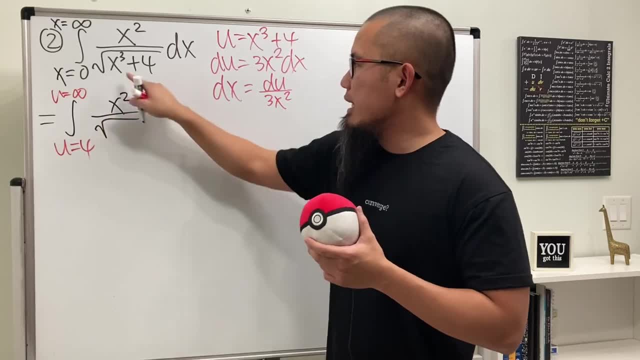 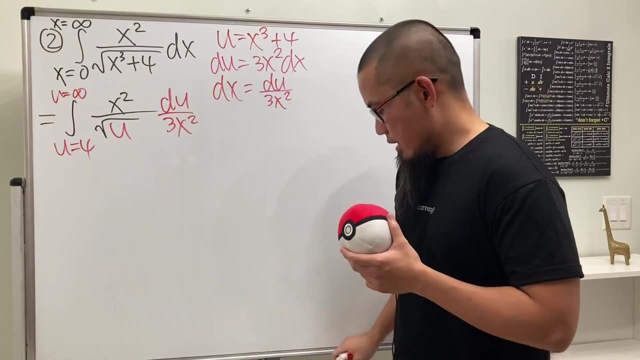 we have x squared over square root, and then this is the u and then dx is that, which is du, over 3x squared, And this is pretty nice, very nice. This and that cancel. So we can just deal with this right. 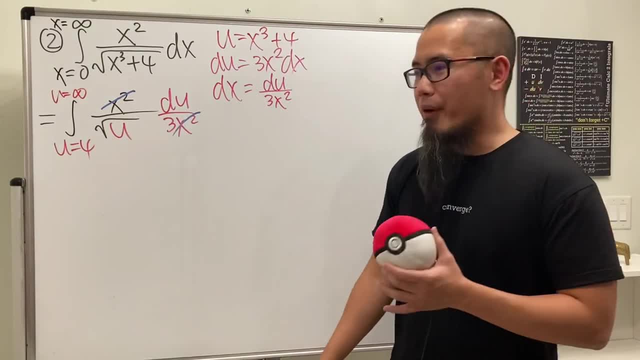 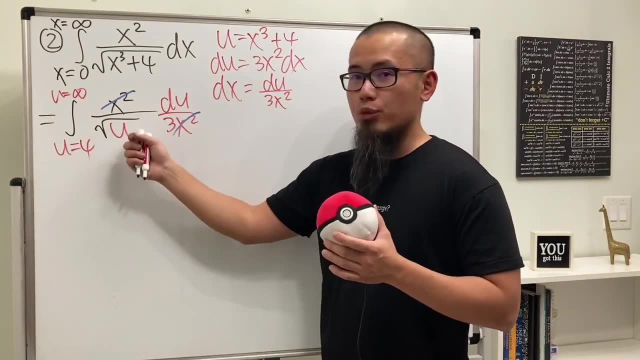 And we'll finish everything in the? u world. However, if you remember the p integral, you should see that this right here does not converge because we have u to the 1 over 2 power. on the bottom p is less than 1, right, So it does not converge. But let's just say we don't. 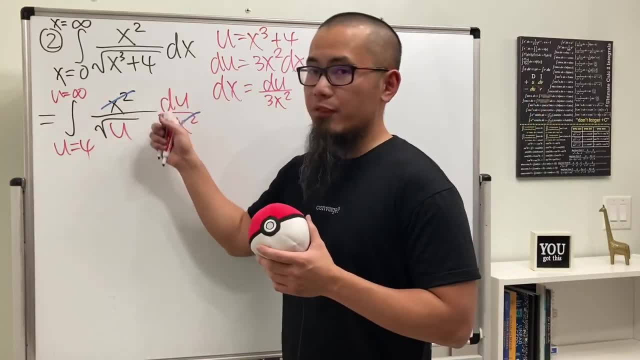 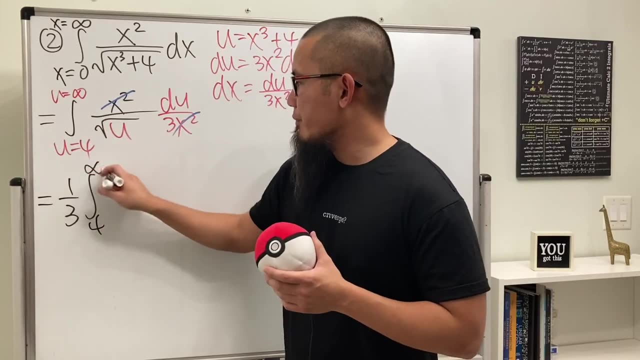 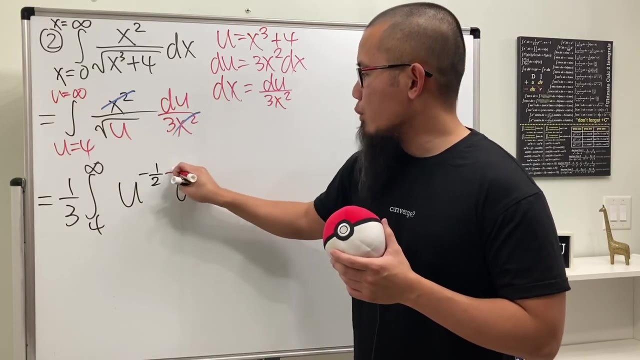 know that. Let's just compute it and see what happens. We have 1 third. put it on the outside, and then we have the integral going from 4 to infinity. The bottom it's the same as u- to the negative 1 half and then add 1 to the power which. 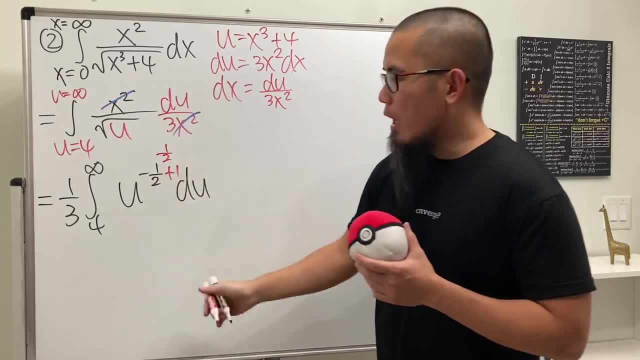 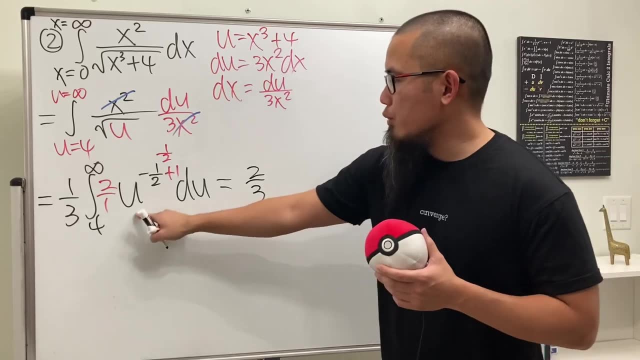 is going to give us 1 over 2, divided by the new power, which is the same as multiply by 2 over 1.. So we get 2 over 3, and then we have u to the 1 half power, and that's just. 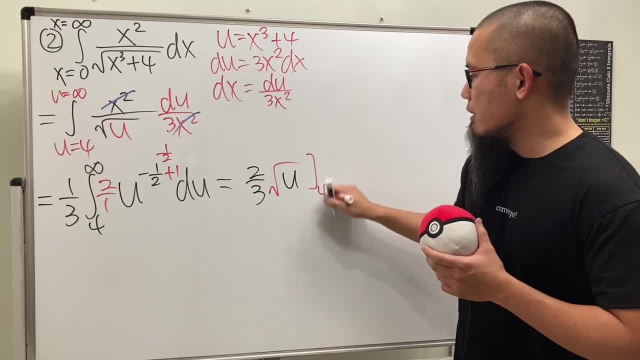 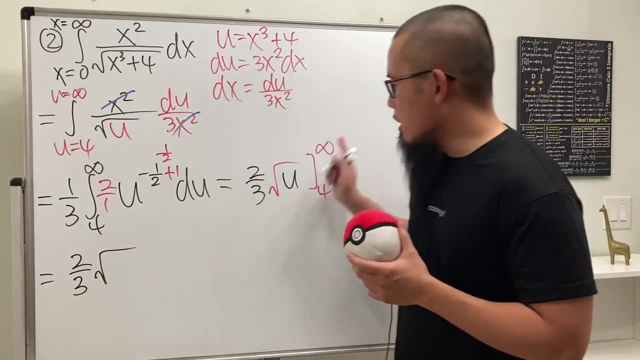 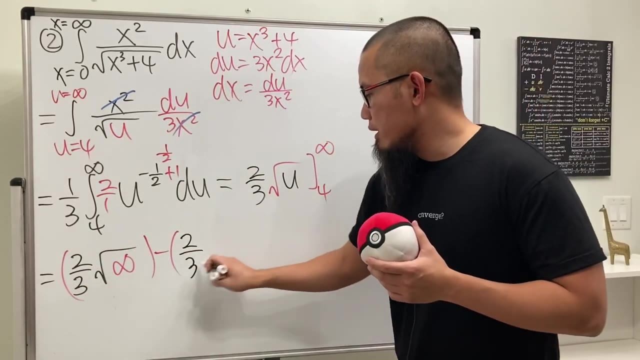 square root of u And then we will plug in, plug in the 4 and also the infinity. When we do that, we get 2 third times the square root of infinity. This is the first term and then, minus plug in 4, we get 2 over 3, square root of 4.. 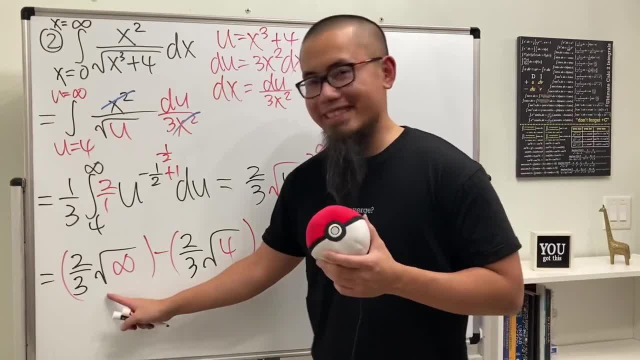 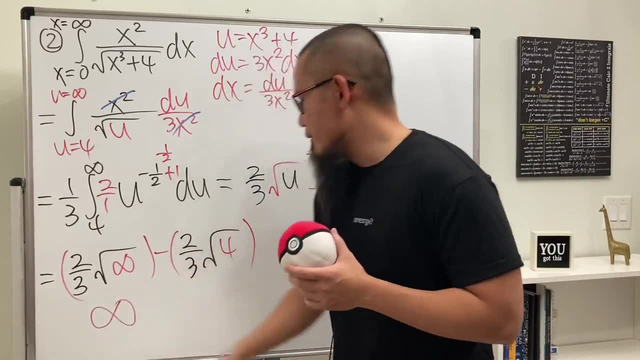 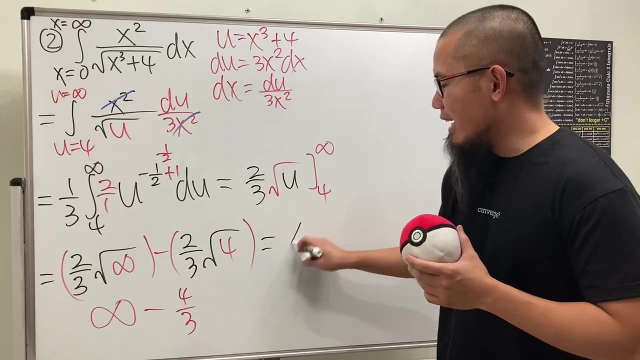 We can calculate this easily, but what's this? Square root of infinity is still infinity. 2 third of that is still infinity. So in fact, here we have infinity minus 4 over 3.. But guess what? This is still infinity, And you can say this right here: diverges to infinity. 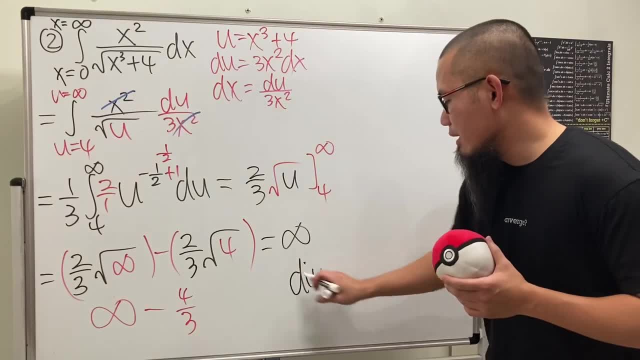 that's okay. But if we do that, we get 2 over 3, minus 4 over 3, minus 4 over 3, minus 4 over 3, but I will just say this right here: diverges, And that's all. That's all you have to mention. 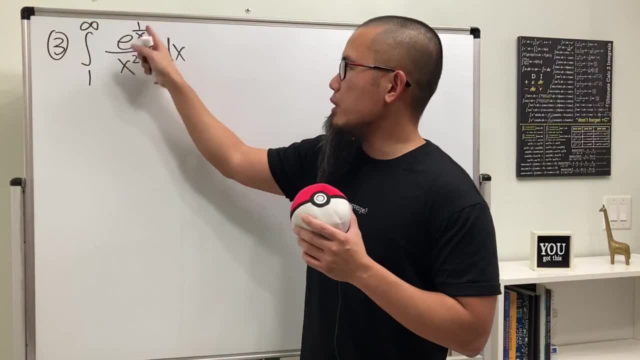 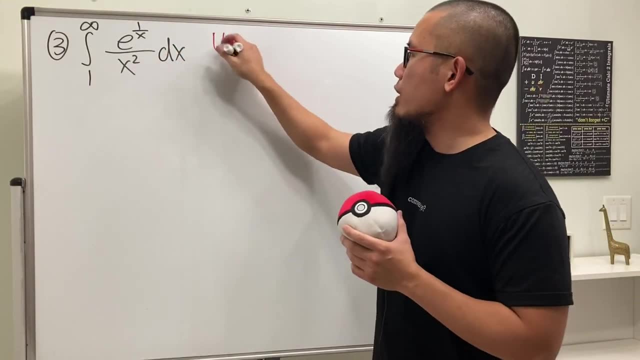 For number 3, we have the integral going from 1 to infinity of e to the 1 over x power over x square. Can we do this up? Yes, Then you equal this guy. so let's go ahead and put that down And we can look at this as x to the negative 1 power, because that way, when 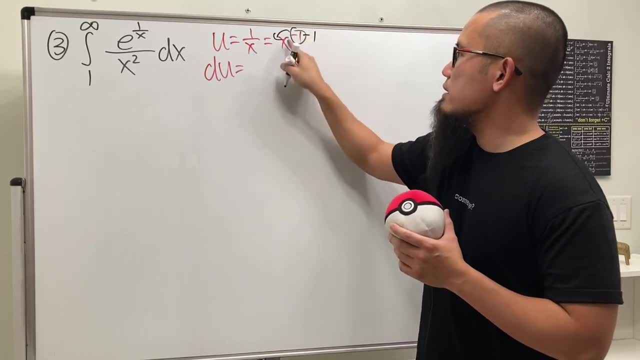 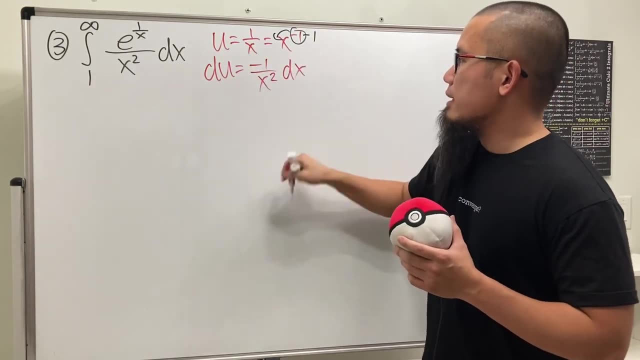 we differentiate- well, we see this right here- will give us negative 1, and then x to the negative 2 power, which is the same as over x square. All right, and then perhaps we can multiply both sides by negative x square, so we get: 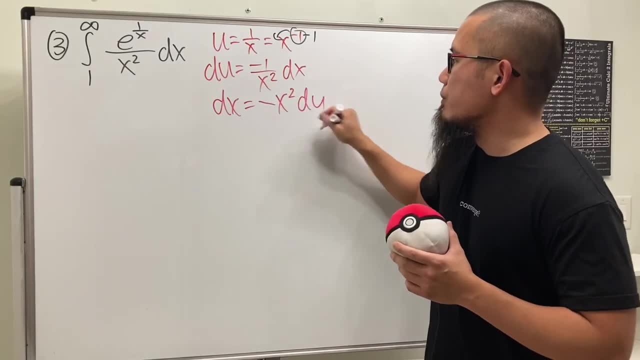 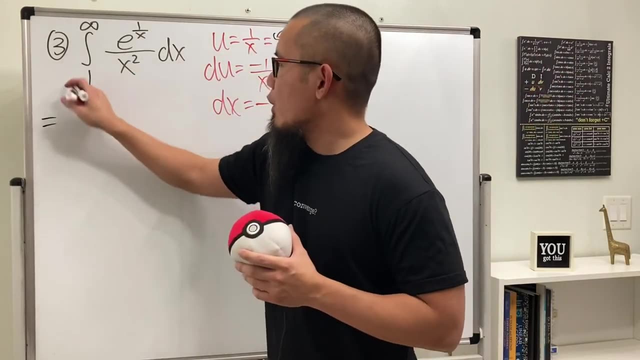 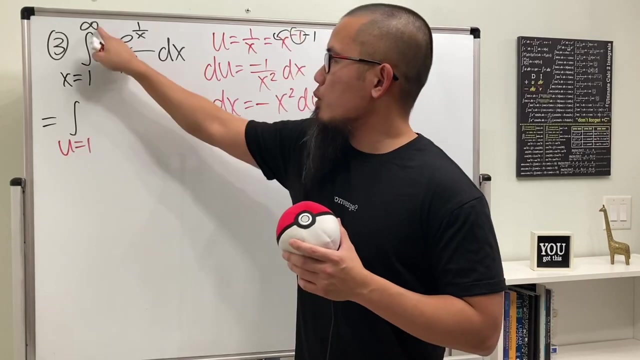 dx equals negative x square du. So this is nice, because now we can go to the? u world, the happiest place for integrations. Here, when x is 1, put it here 1 over 1,, we get 1, so that's a starting for the? u. And then when we put infinity into x, here 1 over infinity. 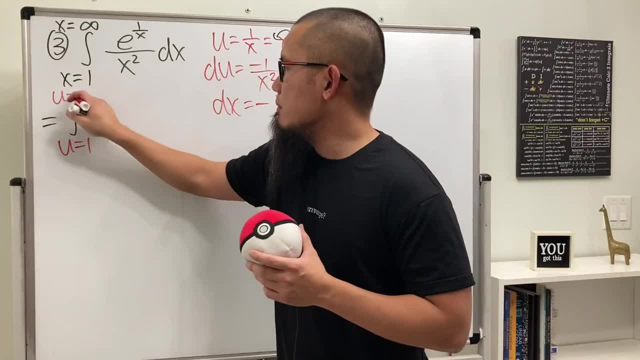 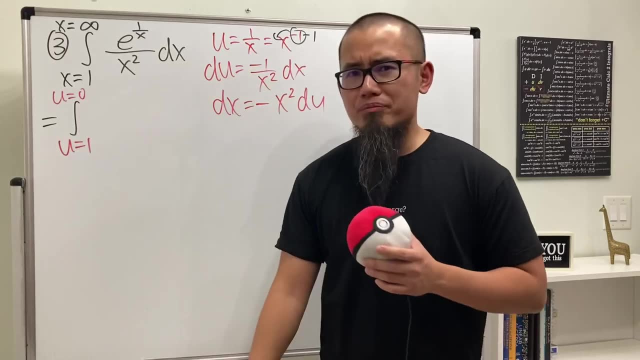 goes to 0. This is weird. 1, 0. Isn't it? usually we have like a smaller number here and then a bigger number here. Right, Okay, we'll see This right. here is e and then 1 over x is. 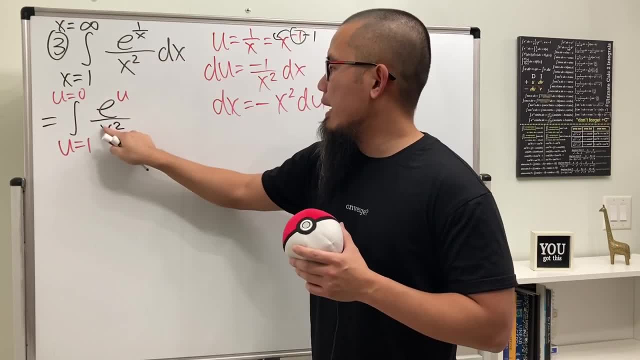 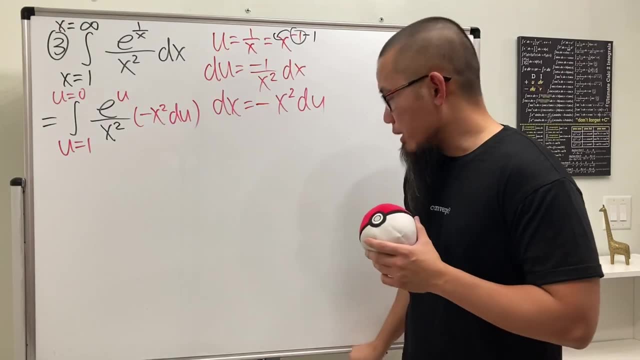 the same as u. and then we have over x square and we see that dx is just equal to that, which is negative, x square, du. So now we can cancel out the x square, which is very nice. But notice, we have this negative here. 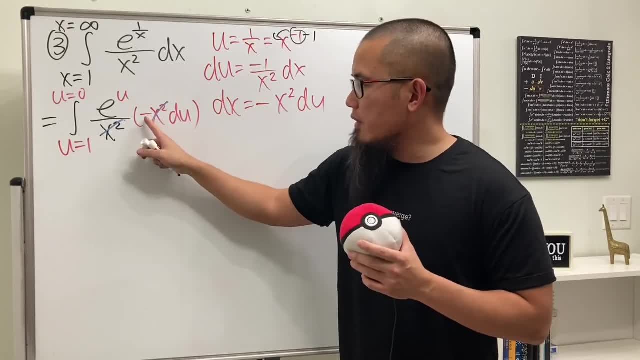 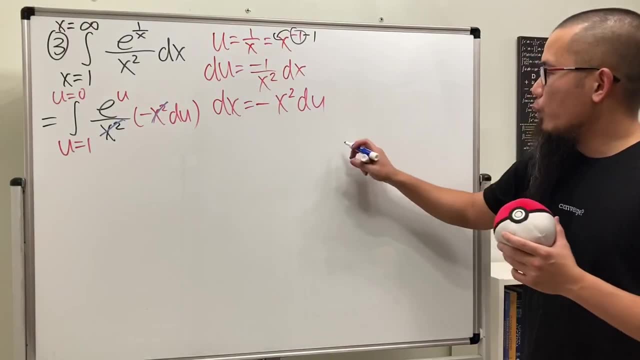 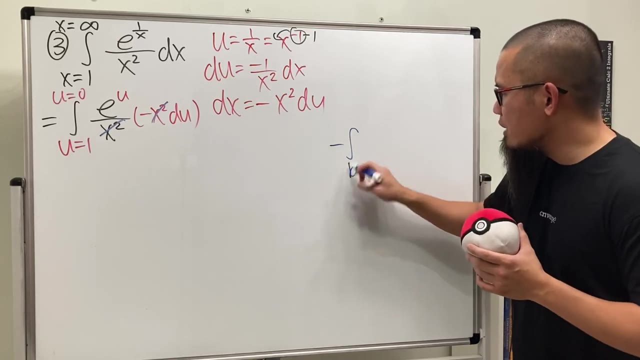 It's kind of useful because in fact we can use this negative to switch these two numbers. What I'm trying to say is the following: Have a look right here. If today we have a negative integral, suppose the numbers here are like out of order. Let's say we have b to a and 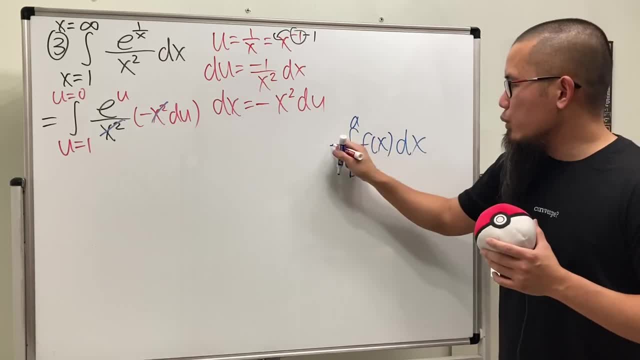 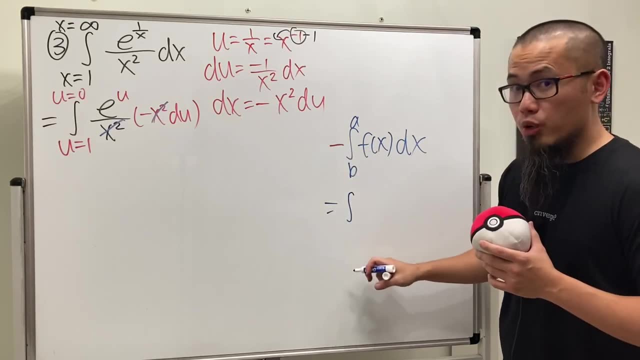 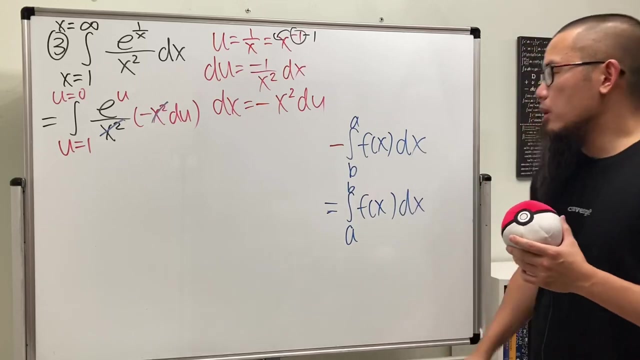 then f of x. In fact, we can use this negative to change these two numbers. We can just go ahead and say this is actually the same as the integral going from a to b, So we can use a to b and then f of x. Why? Because remember, when we integrate this meaning. 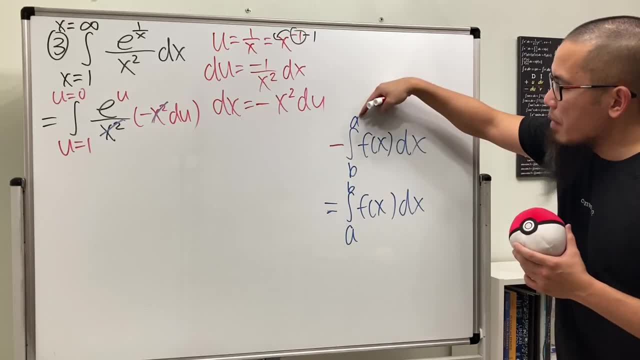 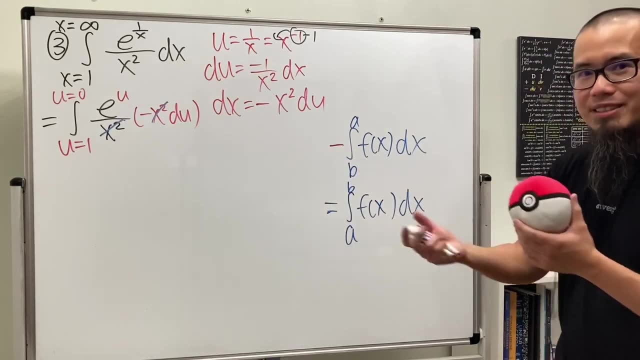 to find an antiderivative for this. we plug in the top number first and then subtract the bottom number. Right We plug in the b, But if you have a negative it's just like the opposite order of the subtraction. So that's pretty much the idea. If you don't. 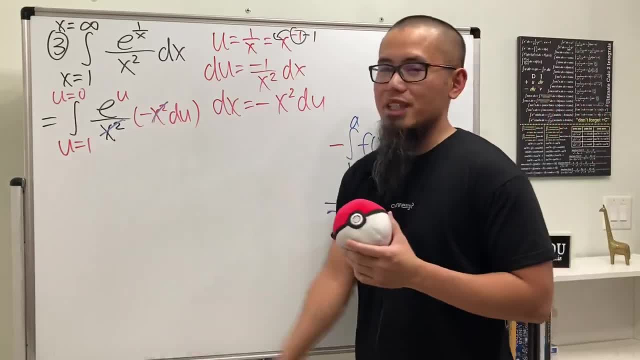 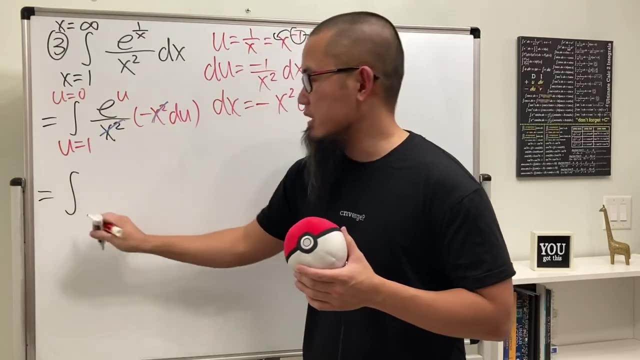 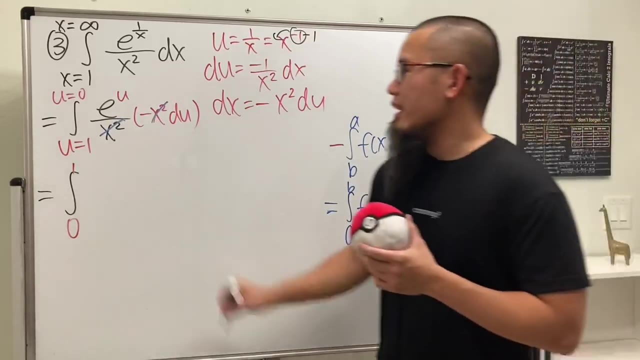 want to do this, it's totally okay. You just have to deal with this negative. But enough on that one. I'll use this negative and change the integral, going from zero first to one. I'll switch this and I don't need to put on a negative anymore because of that. And then here we have just 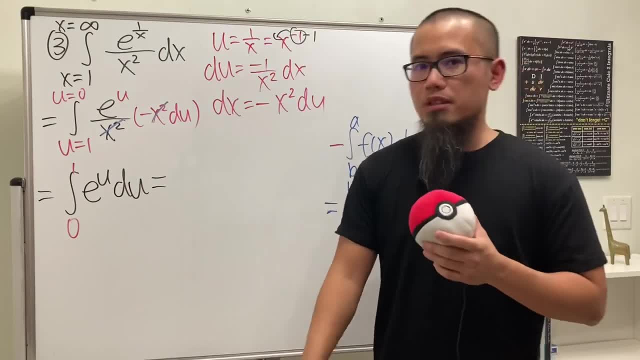 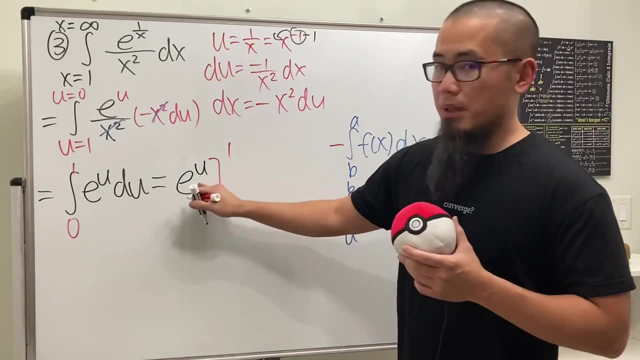 e to the? u du. and now let's finish everything. in the? u world We get. well, integral of e to the? u is just e to the? u. and then we have to plug in. This time we plug in one first. You see, We plug in one first: e to the one. 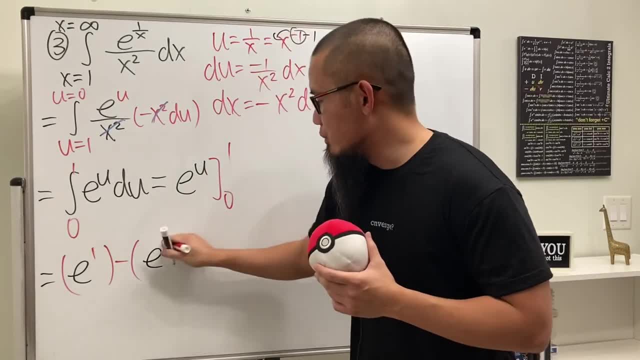 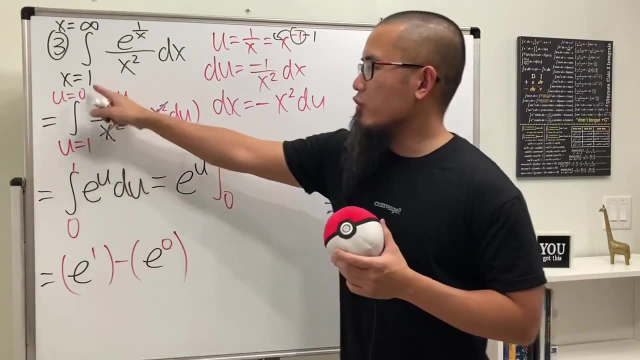 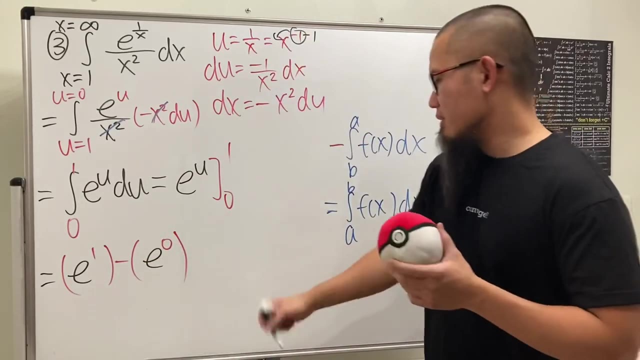 And then minus e to the zero. Oops, wrong column. If you didn't switch the order of integration, then you have to plug in zero first, and then minus, plug in one, And then you have the negative on the other side. So it's just a different order, But you know. 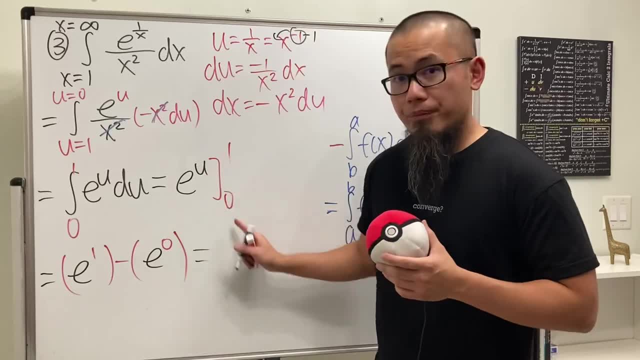 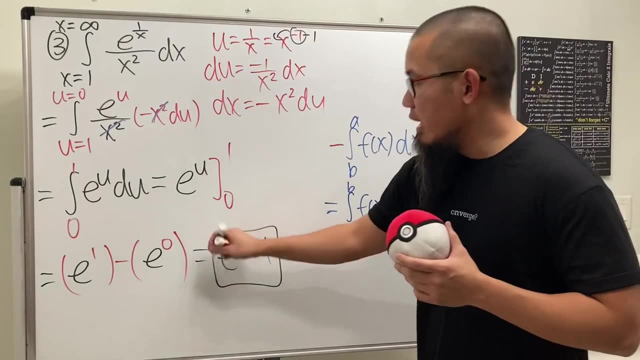 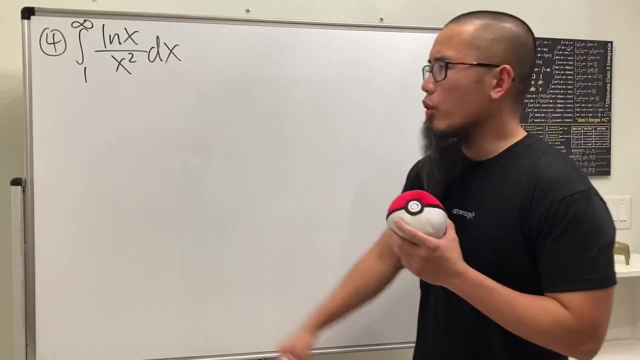 in the end you end up with the same answer. Be really careful, though. Plug in zero here you end up with one. So the answer is e minus one, And this integral does come first and converges to e minus one Number four. we have the integral going from one to infinity. 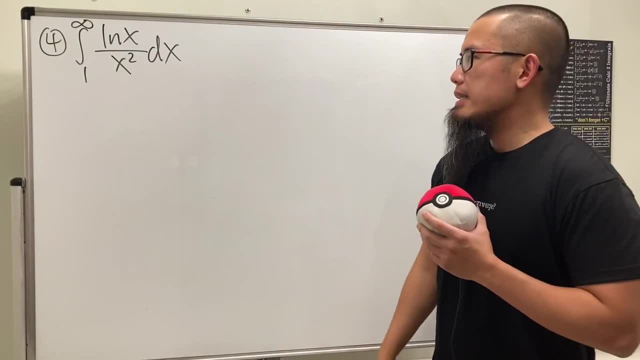 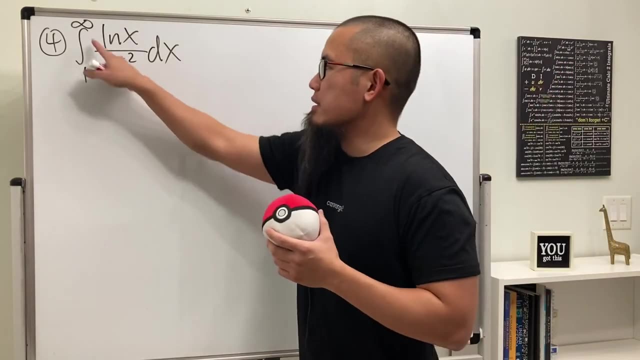 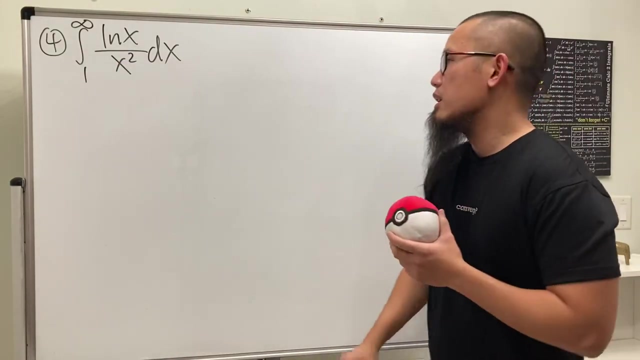 ln x over x squared We cannot do use of anymore. In fact we will have to do integration by parts, because this is the same as x to the negative t2 power and then times ln x. That's one of the forms that you should know that we do integration by parts. So of course let's put it down on the 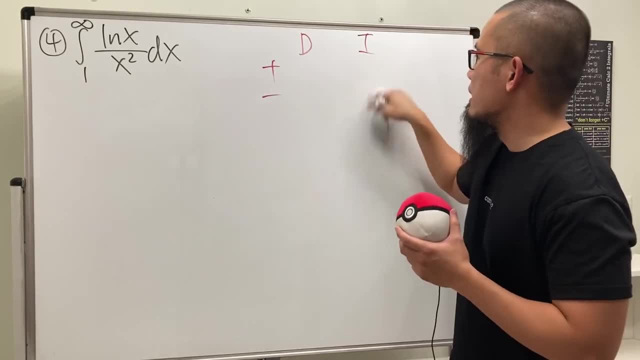 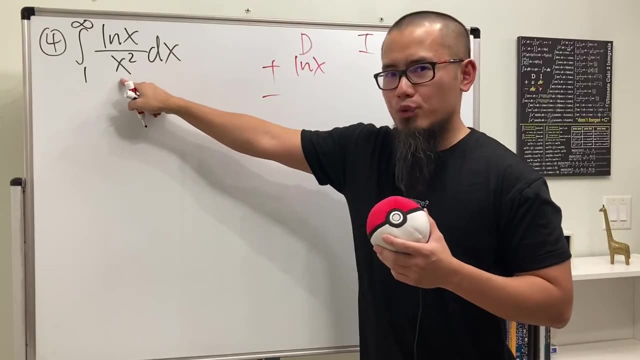 side d and also the i plus minus. Let's go ahead and differentiate ln, x And then integrate. well, not x squared, but rather one over x squared right, Which is the same as x to the negative t2.. All right, make this happen. 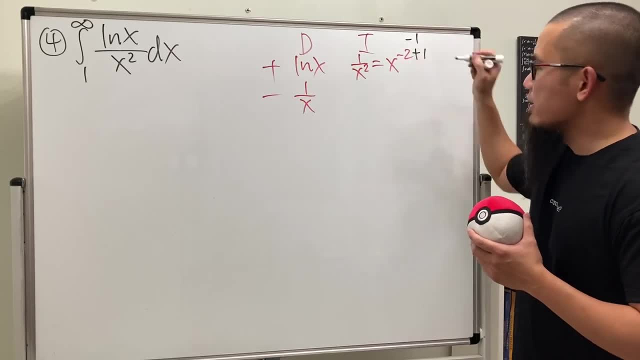 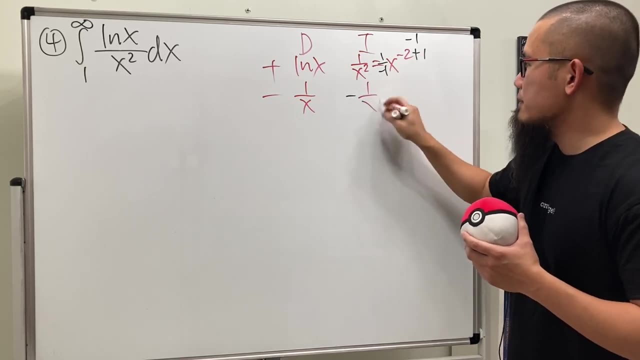 We get one over x. Make this happen: We add one to the power which is negative, one divided by the new power. So we get negative and then x to the negative one, which is just one over x. So now you see, this times this is the first part of the answer. So we have. 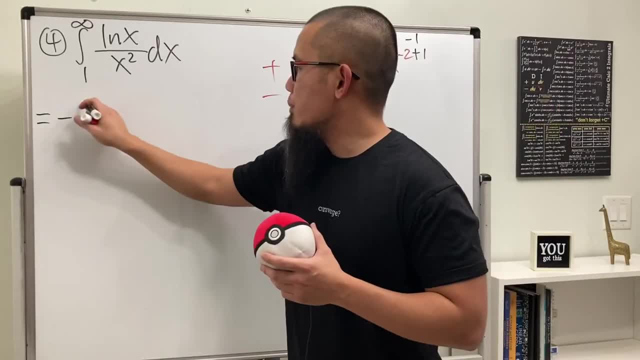 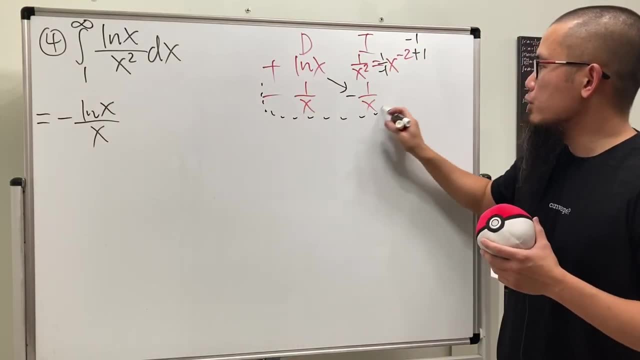 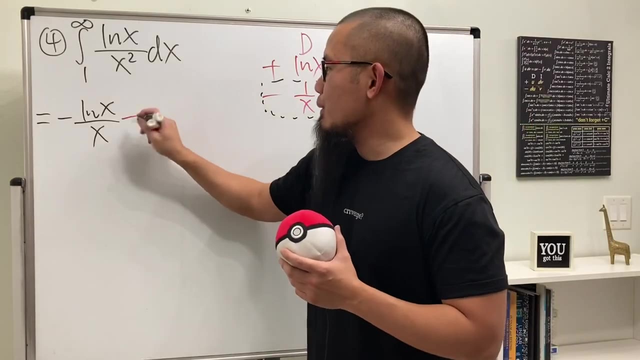 negative. and then let's put down ln x over x. And then don't forget that we will have to multiply these two things together and put that inside for integral. Negative times a negative, we get positive. And don't you guys just miss that? Back in that pre-algebra the teacher said: 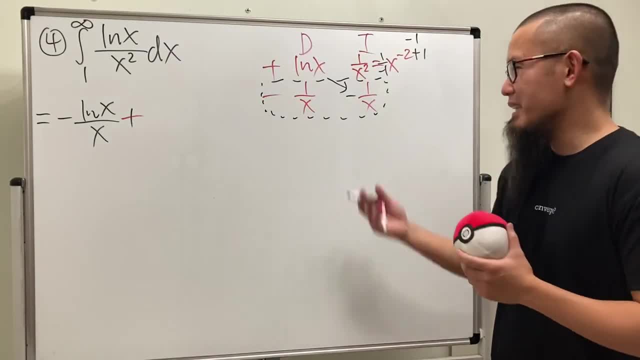 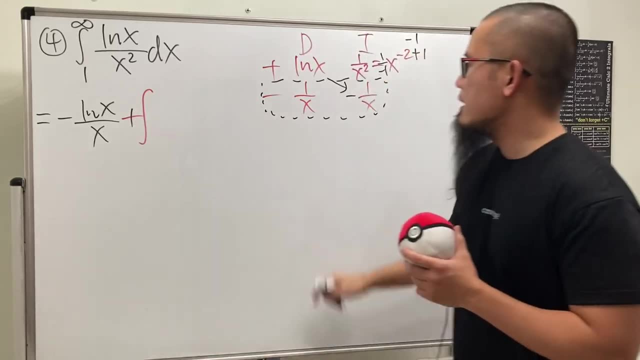 negative times. negative is a positive. That's all you have to learn, right, Good old days. But anyway that. and then, don't forget, we still have to put down an integral, And then one over x times one over x, which is- let me just write it down for you guys: 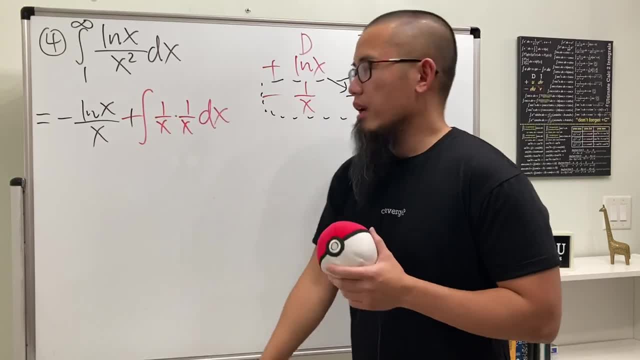 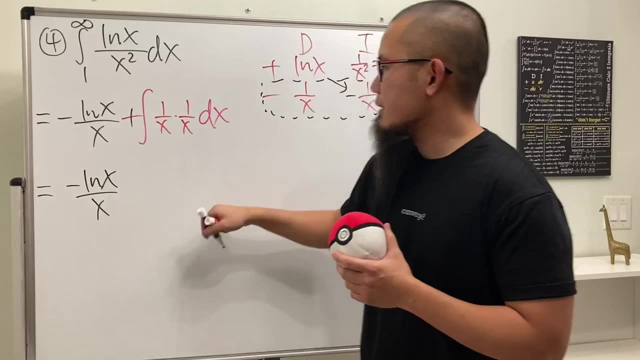 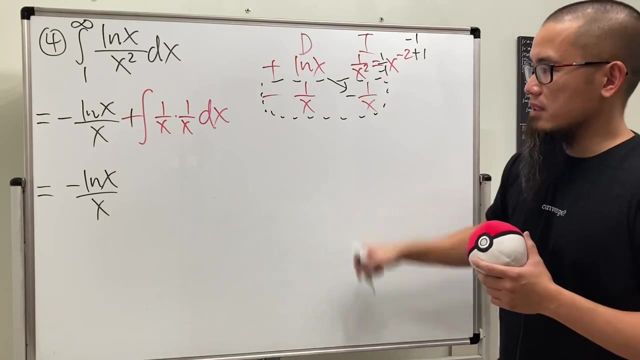 just to show work nicely, like so, And let me just finish this right here real quick: This is still negative ln x over x. And then this is the same as that right One over x squared. we have to integrate that. We get negative one over x. So work that out. You get negative one over x. 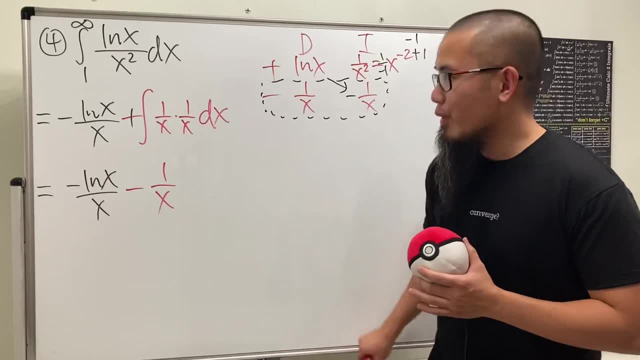 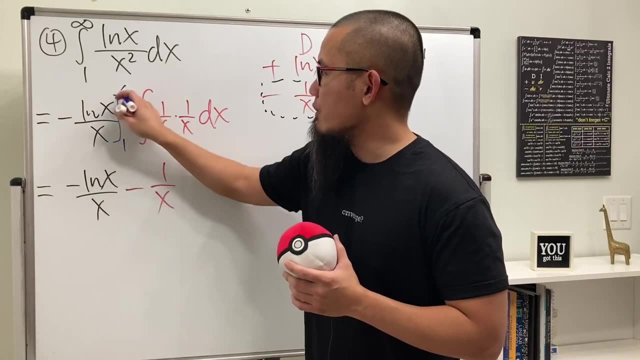 We're not done yet Because, remember, we have the limit of integration. So, right here, 10 equal d. I should have put this down. We go from one to infinity, And right here, I should have still put down one to infinity. 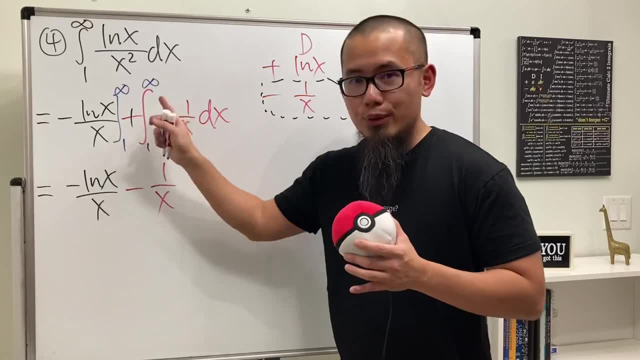 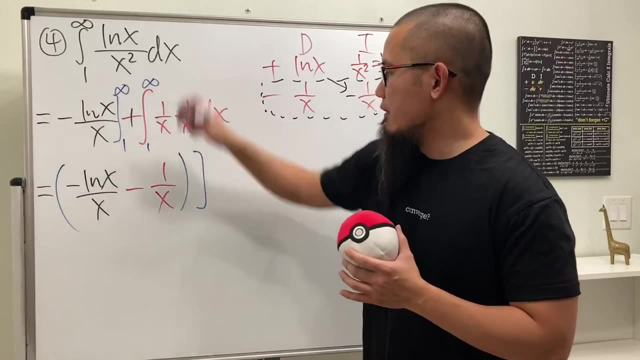 But what you can do is just ignore that for now. Just do the integration by parts, And once you finish all that, and then you plug in the value right one and also the infinity. Here's the d, although When you put infinity to here, 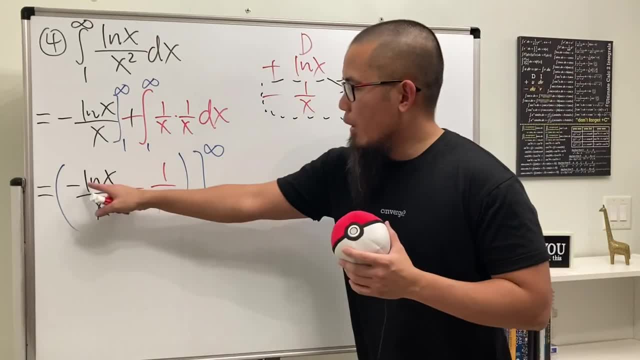 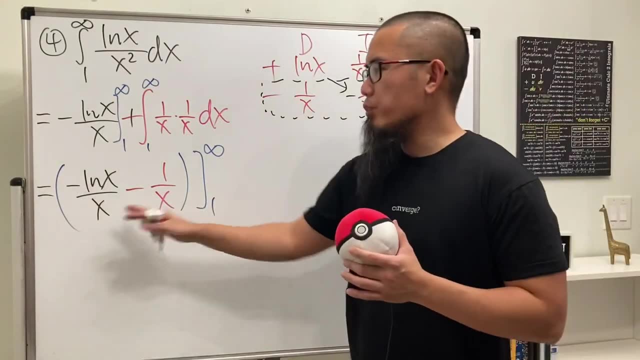 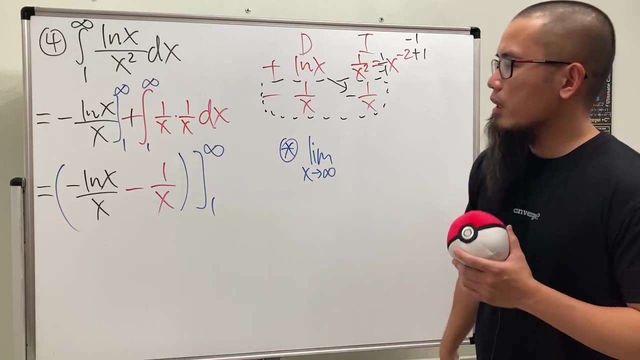 what do we get? Well, ln infinity is infinity over infinity. That's technically indeterminate form, right? So we should technically put that on the side. So I'm just going to make a note on the side. If we take the limit as x goes to infinity, we do have a negative. You can put it down. 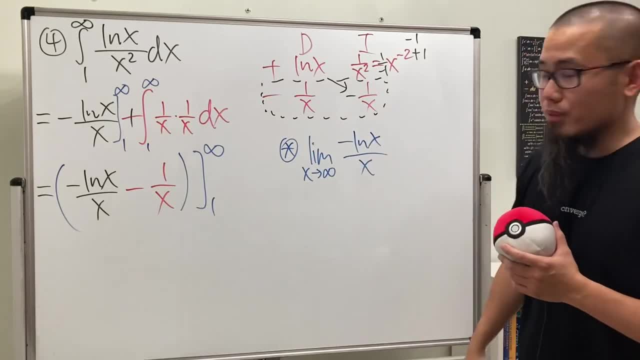 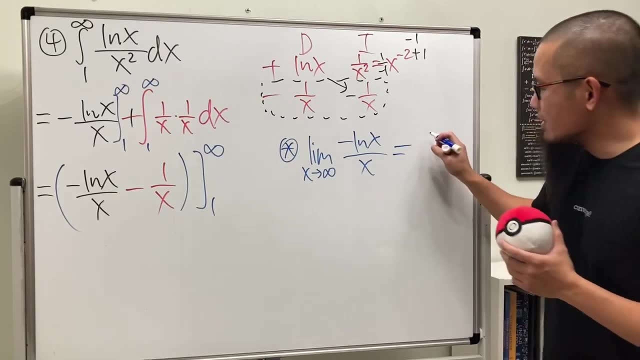 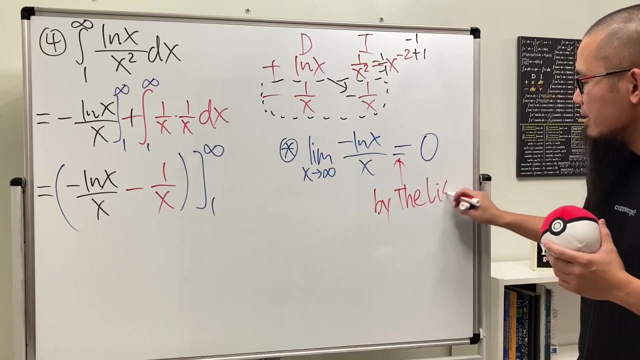 Or not Doesn't really matter, because the answer will be zero. Well, what's this? What's the answer for this Zero? How come, Why is this zero? Why is this so easy? Yes, in my class you can just say by the list. That's why. 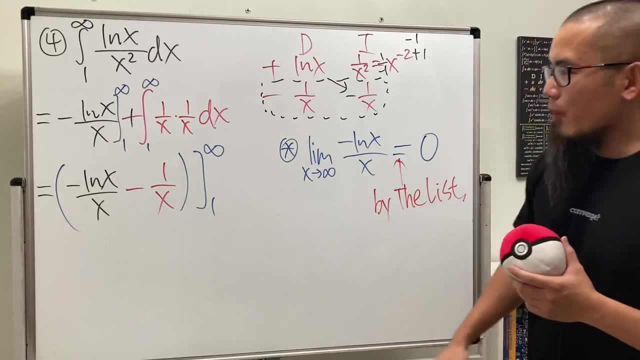 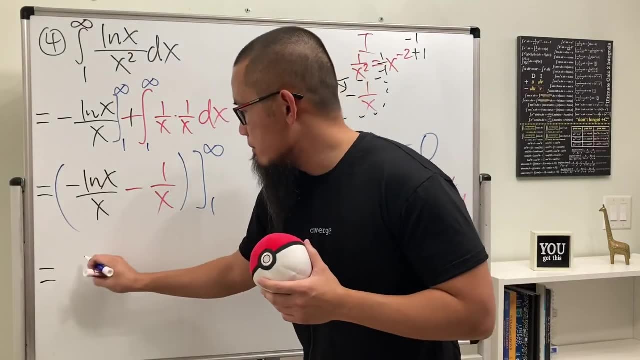 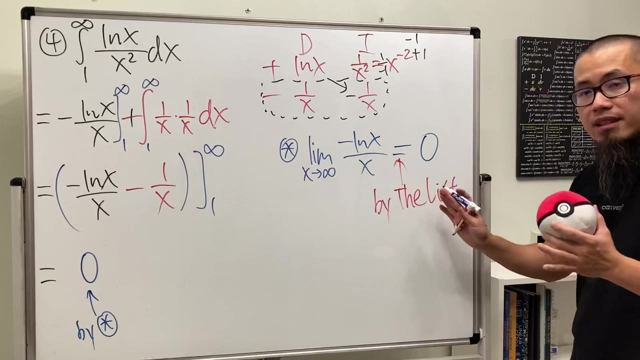 I went over all the secret weapons with you guys. So when we put infinity to here- I'm just going to write it down right here for you guys- We get zero. And then, if you would like, you can just say by star, which is just a supplement on the side that you have to provide, And then what you can. 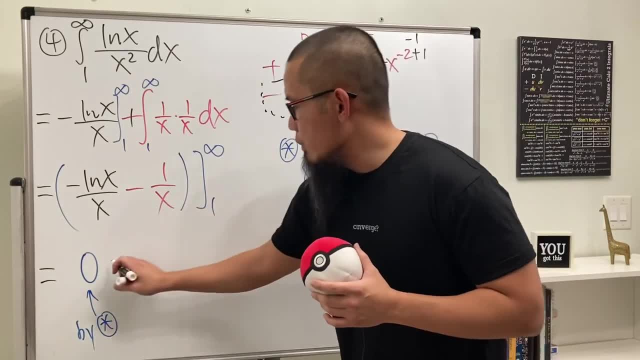 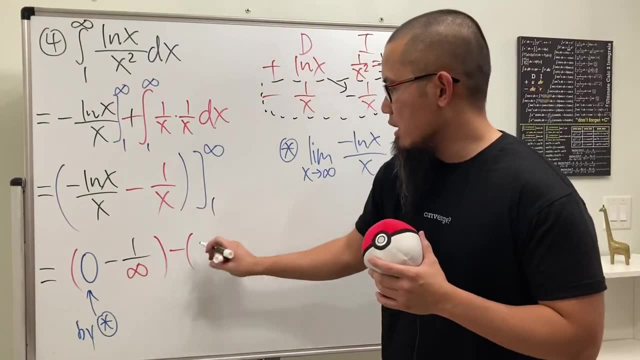 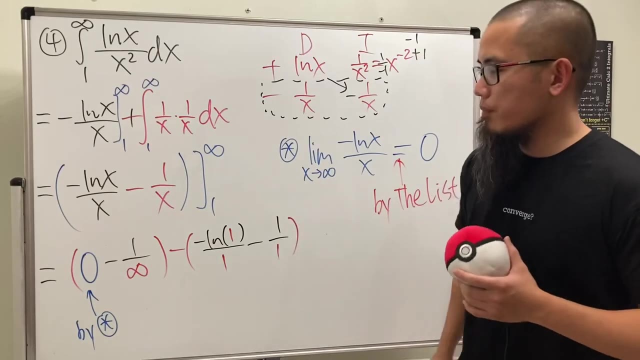 do is put the rest, Put infinity. here We have minus one over infinity, And then minus, put a one, put a one, all that right. So we get negative ln: one over one, minus one over one. Okay, By the way. 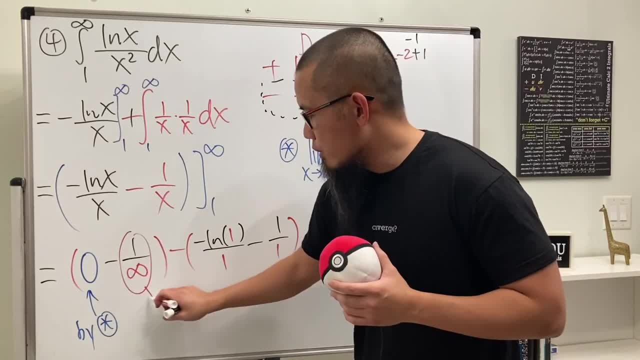 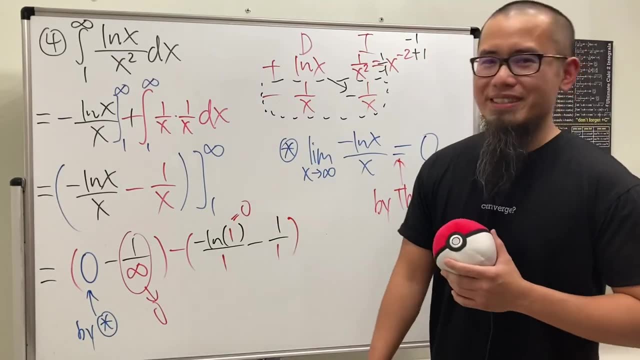 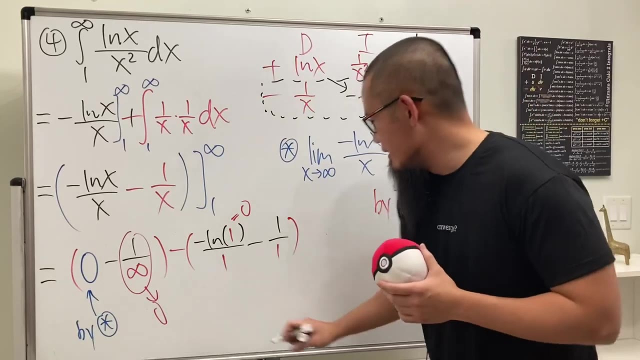 this right here is zero. Guess what This guy also goes zero. because we can draw a conclusion nicely: ln one is zero, So that's also good. Finally, people negative, negative one, Negative times, negative one is positive one. So the answer for this is just: 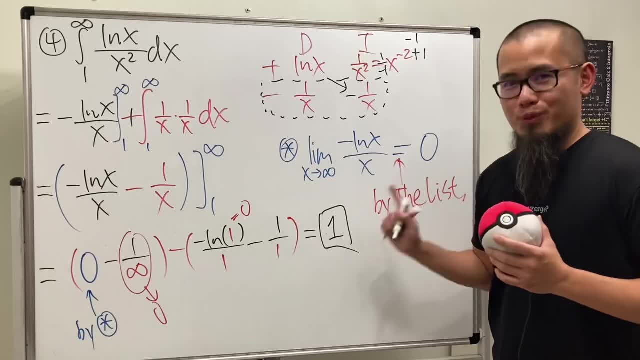 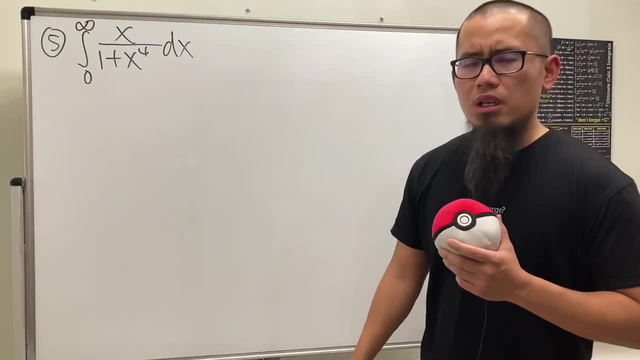 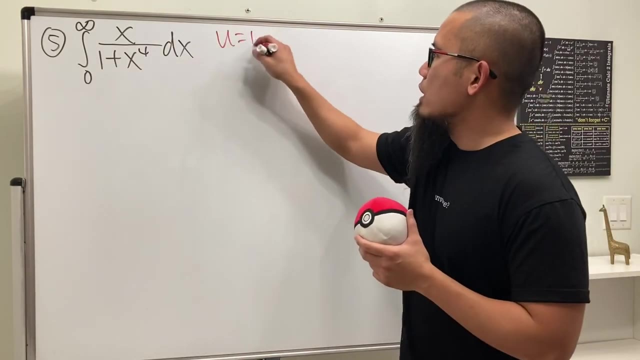 positive one. All the work for one Number five. we have the integral going from zero to infinity, x over one plus x to the fourth power. Do we use u substitution? Yes, Should we let u equal the bottom? Let's see. If we do that, we'll differentiate both sides. We get: du is equal to four, x to the. 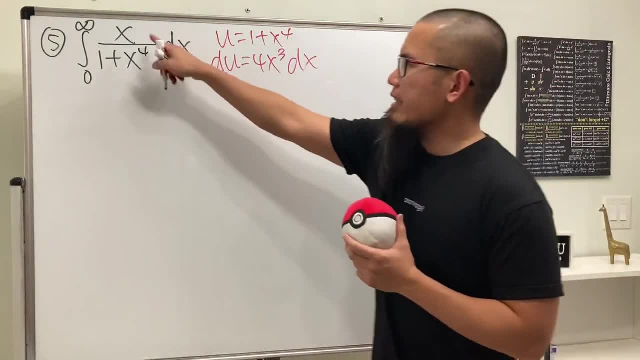 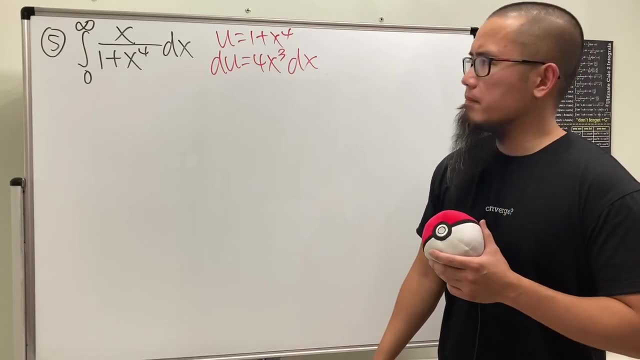 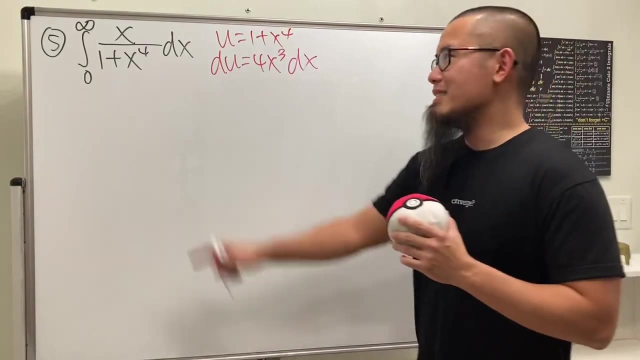 third power. dx On the top. we only have x to the first power. This is four x to the third power, So they won't cancel each other nicely. Did I just make a mistake on the homework? Should this be x to the third power? No, I did not. It's meant to be x to the first power. 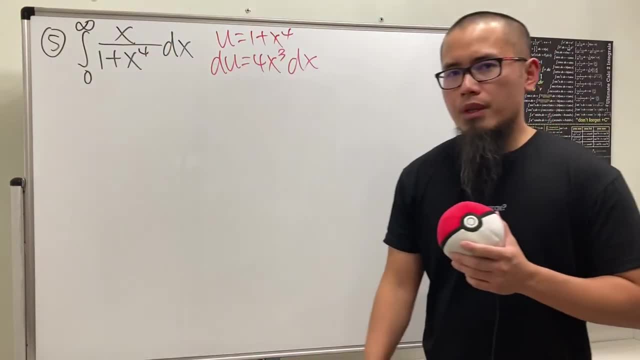 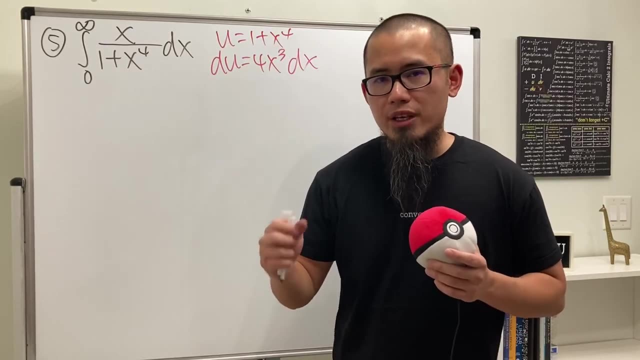 Well, think about it. If this is x to the first power, u should be what Something x to the second power? Because that way, when we differentiate the u, we'll get something x to the first power, right? So do we see x to a second power here? 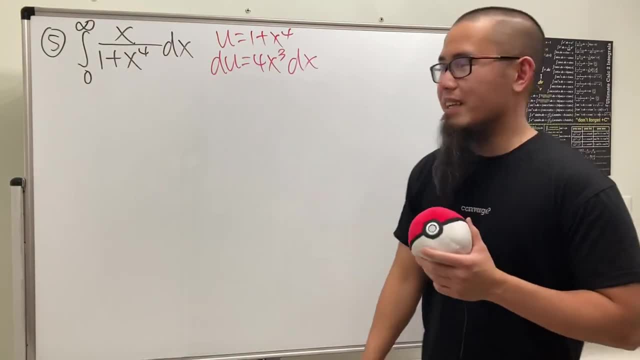 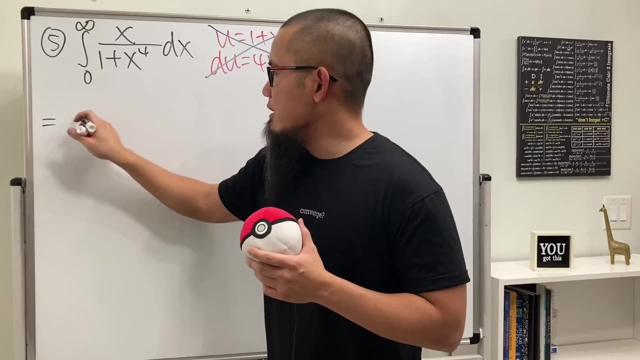 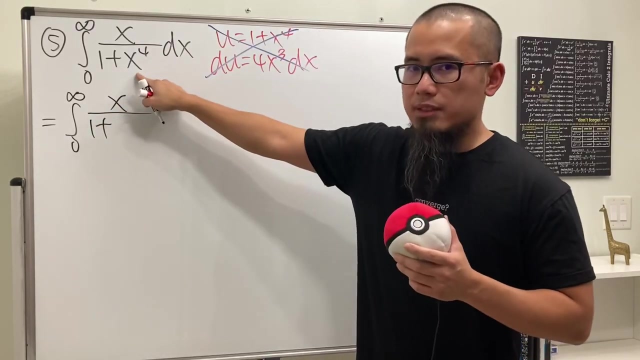 This is suspicious. huh Yeah, that's the key right here. So we don't do this? u right here. Here's the deal. We look at this integral going from zero to infinity, x on the top, over one plus instead of x to a fourth power. Let's look at that as parentheses: x squared and then squared. 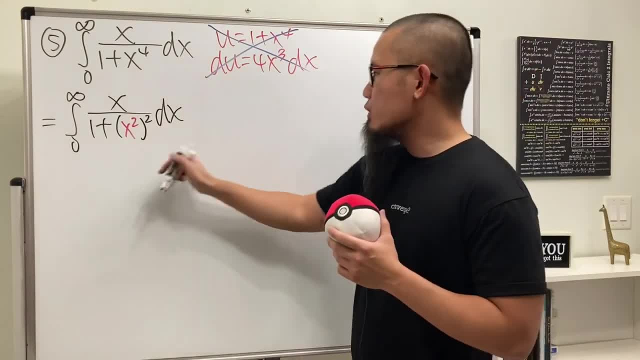 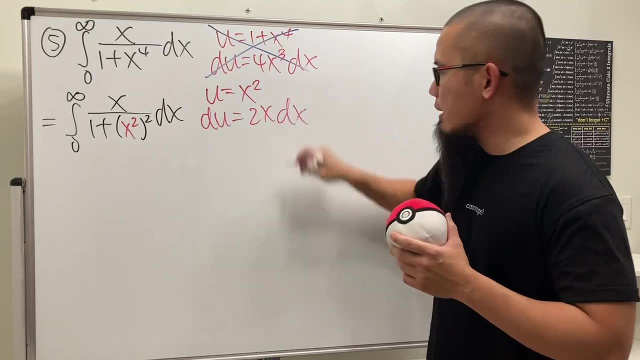 Ah, much better, right? Because this way we can just let u equal x squared And then we see du is just equal to 2x dx. And by now you know, so far I've been telling you guys, maybe let's just divide. 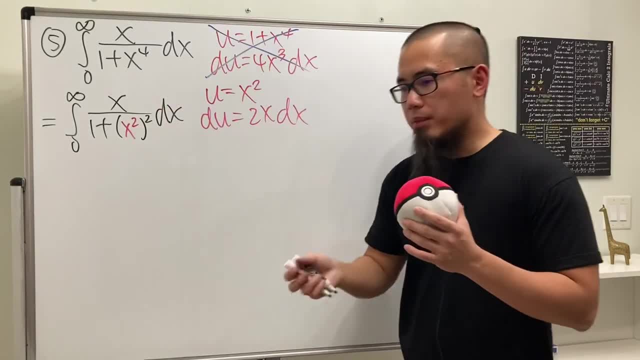 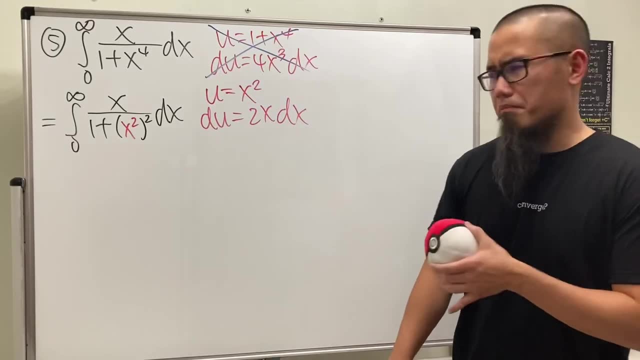 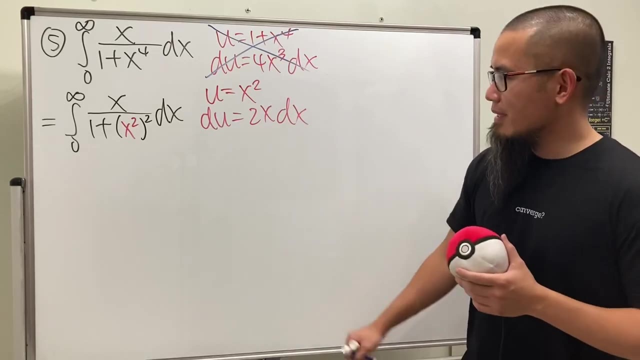 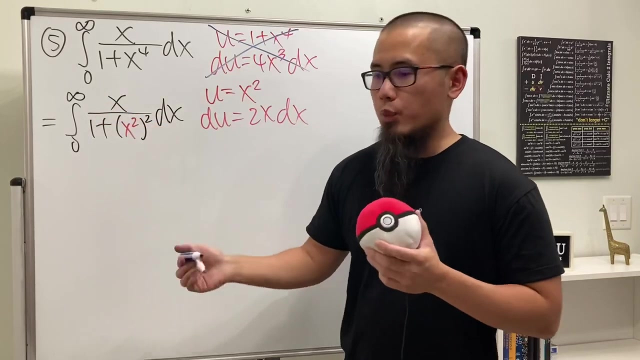 the 2x on both sides, so we can isolate that, so you can see what numbers to divide and things like that. But we have done a lot of that already. I will show you guys perhaps a better way or quicker way. Anyway, we do have the x- dx right here already. What we're missing is just the 2.. So why don't? 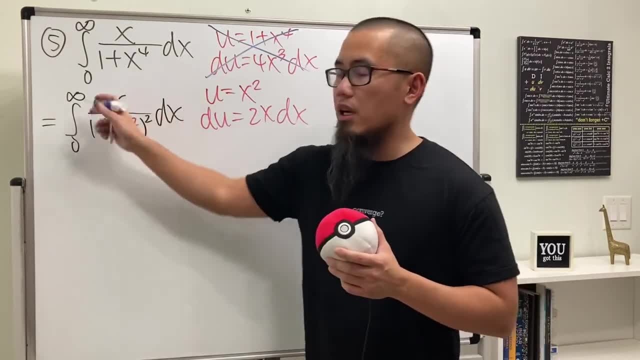 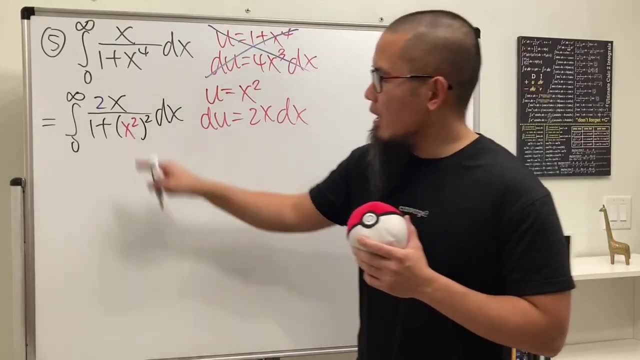 we just multiply this by 2?. So that way we can see the top is just the du. But of course I cannot multiply out the 2 right here out of nowhere. It's okay, When we multiply the 2 right here, just make sure that we divide it by it. That way we still have the same exact expression. 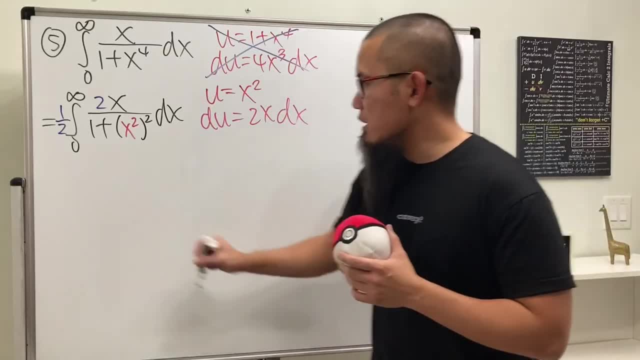 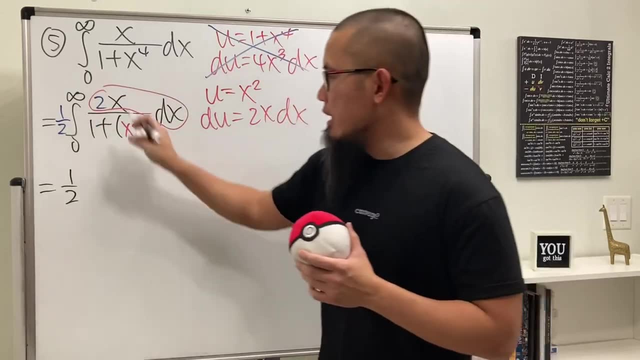 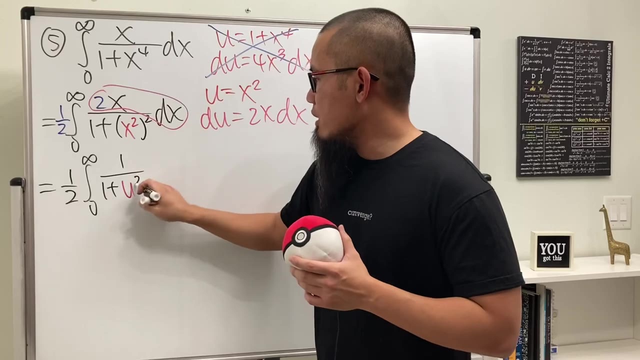 Right. So the beauty of this is that we see we have the 1 half right here right away, And then again this right here is just precisely the du, And then we just have the integral going from 0 to infinity, 1 over 1 plus u squared, And then we have the du on the side. Yeah, All right. And then 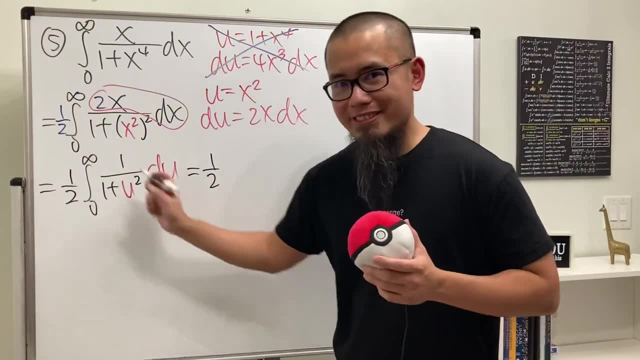 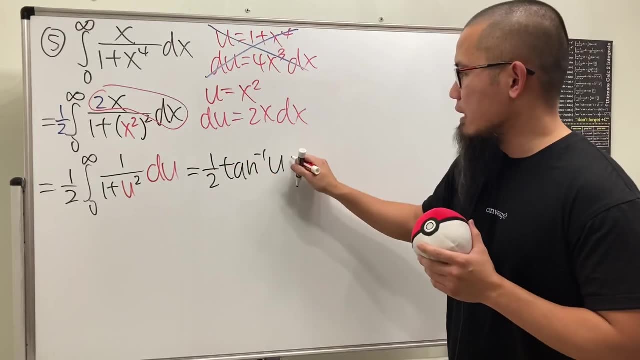 we see this right. here is just 1 half. And what's this? Inverse tangent of u, Yes, So we get an inverse tangent Of u. And then, don't forget, we have to plug in now. So we plug in 0, infinity, Infinity go. 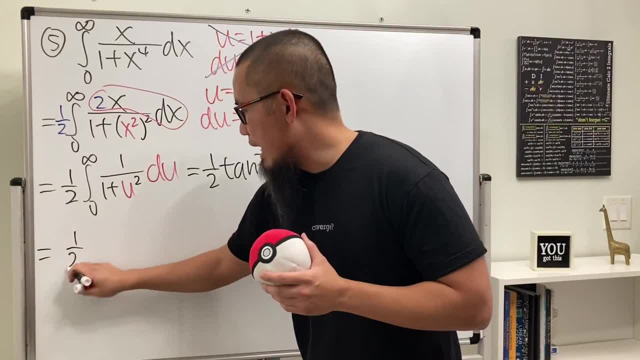 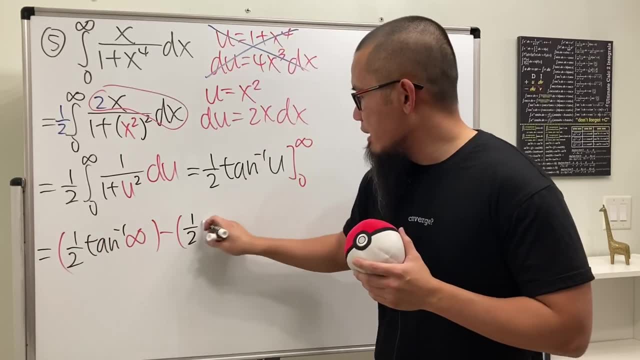 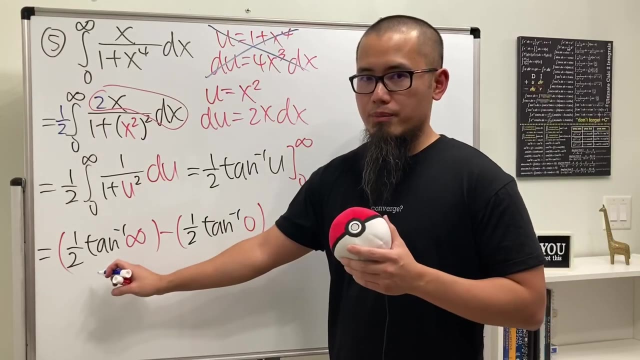 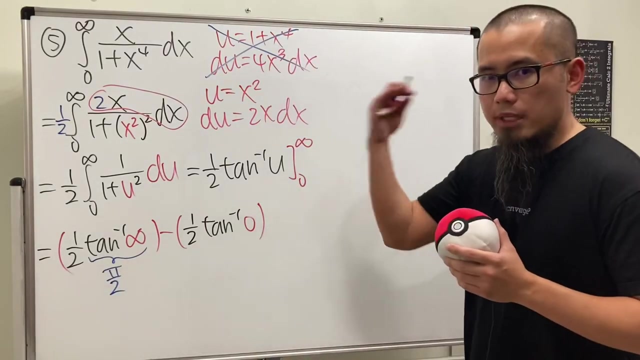 first, So first term, we get 1 half inverse tangent of infinity, And then, minus second term, we have 1 half inverse tangent of 0.. Well, can we draw a conclusion right here? Yes, Inverse tangent of infinity is pi over 2 because of the graph, It has the horizontal axis. 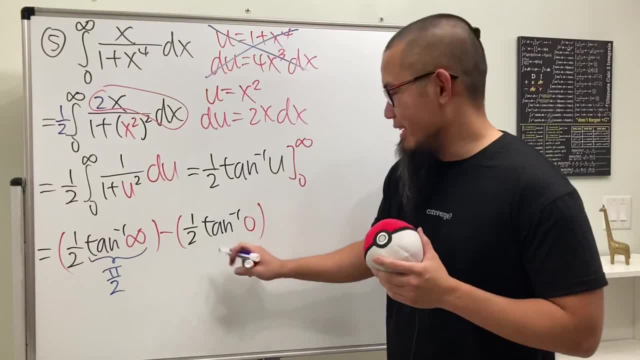 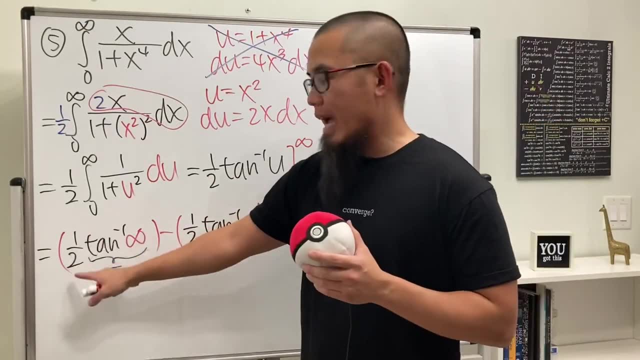 And can we draw a conclusion right here? Yes, Inverse tangent of 0 is just equal to 0. So, as you can see, this is just 0. So we just have 1 half times pi over 2. And that's going to be pi over. 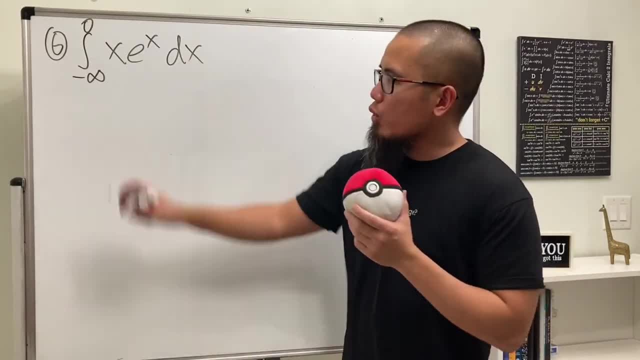 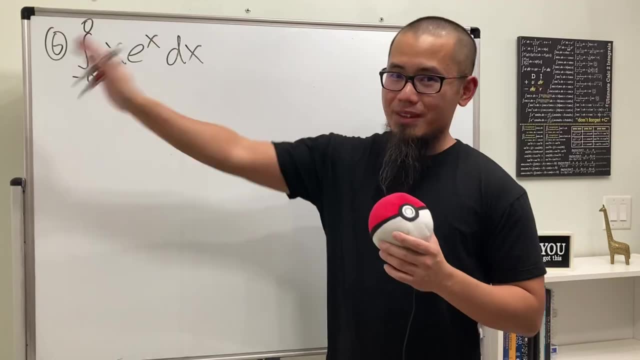 4. For number 6, we have the integral going from negative infinity to 0, x times e to the x. This is still improper. We just have to go from all the way to the left and then to 0, right, So still. 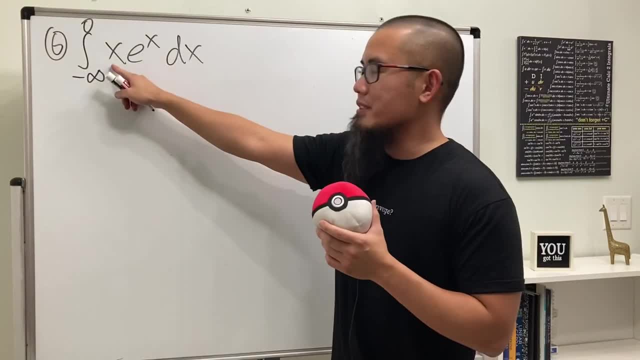 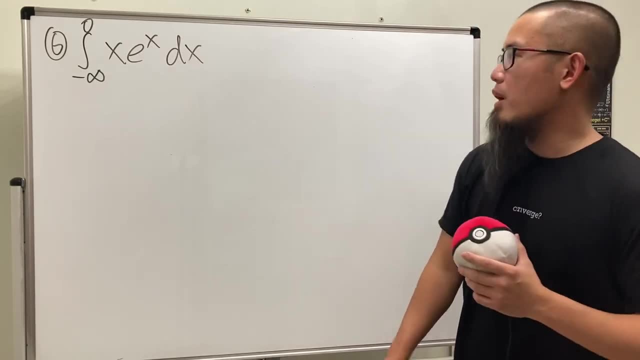 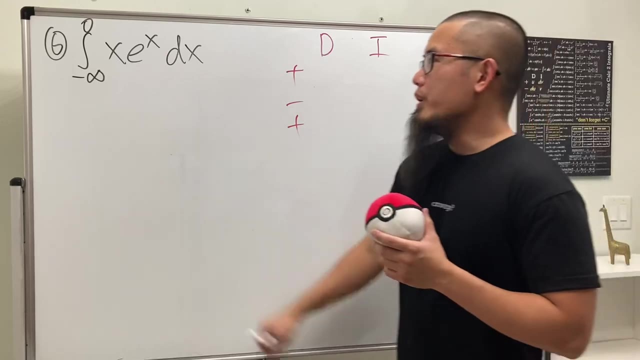 infinite interval. Well, the main question for right now is how do we integrate x times e to the x? Not use substitution anymore, But rather we do integration by parts. So let's put this down on the side. Of course, do the di plus minus plus. We are going to differentiate x and. 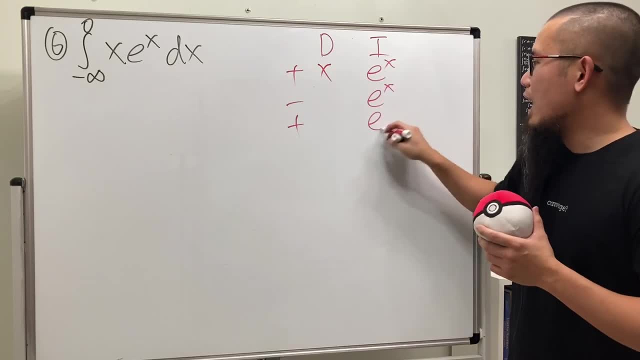 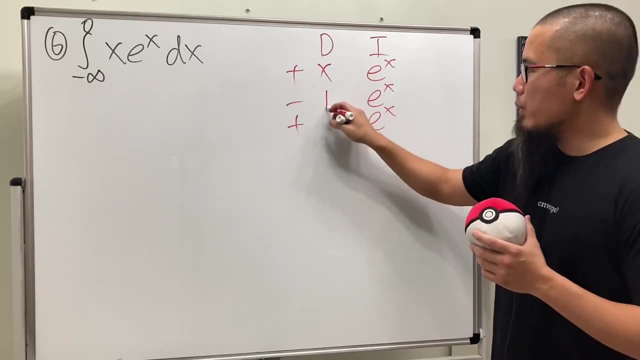 integrate e to the x. We can integrate e to the x however many times as you would like, But don't do that, of course. Just stop right here, Because you know differentiating x. one time we get 1.. Again we get 0.. So we stop right here. Ladies and gentlemen, this times this, this times that, 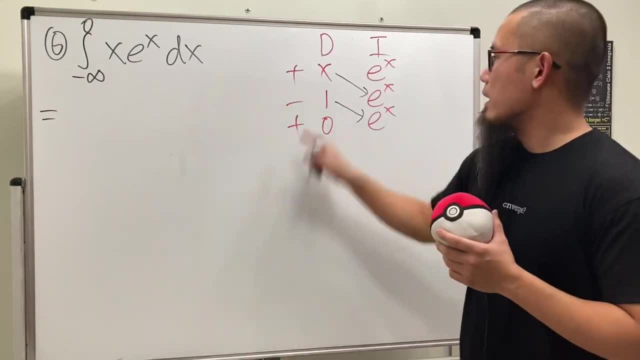 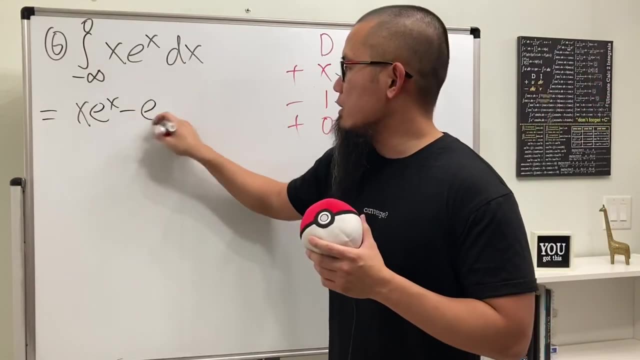 will be the answer right, So we know this right. here will be x times e to the x. That's the first part of the answer, And then second part of the answer is minus e to the x. Okay, then we plug in. 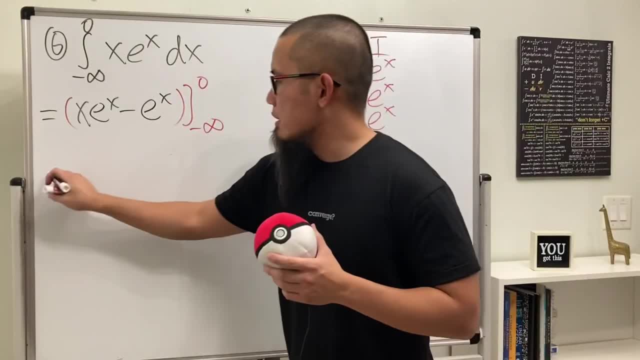 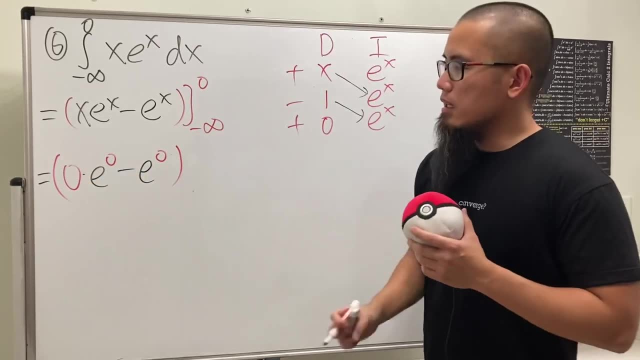 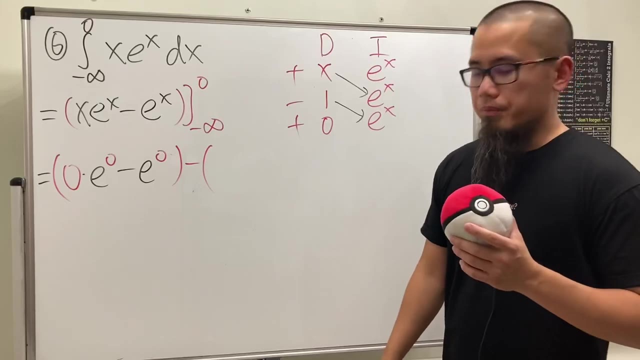 0 first. So we get 0 times e to the 0 minus e to the 0 first. So that's the first part of the answer And then the second part. we just plug in negative infinity and we subtract. But here's a small issue: If we put negative infinity here, times e to the. 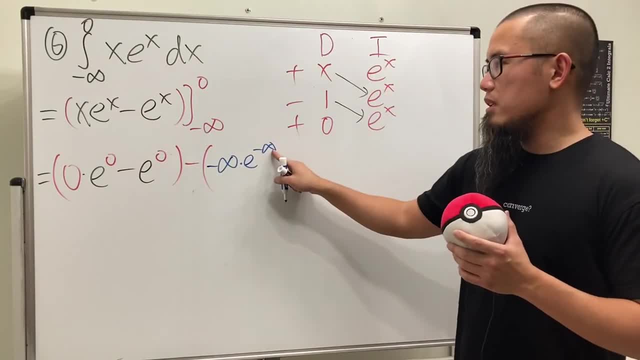 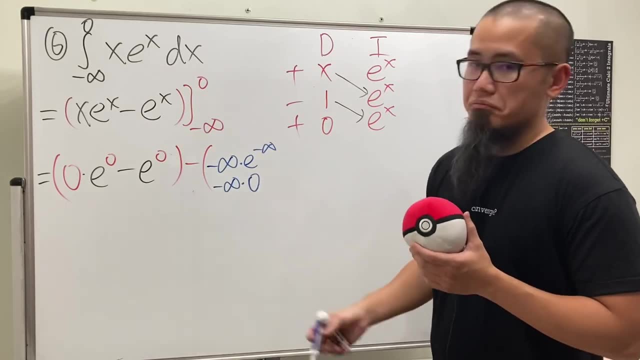 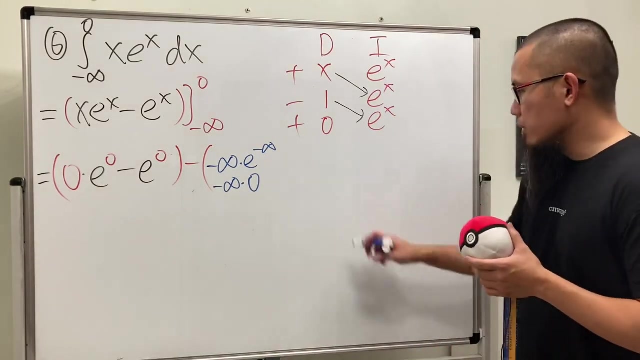 negative infinity. e to the negative infinity is the same as saying 0, right, So this is technically negative infinity times 0.. We cannot draw any conclusion yet. We will have to supply some work on the side, So let's do it. 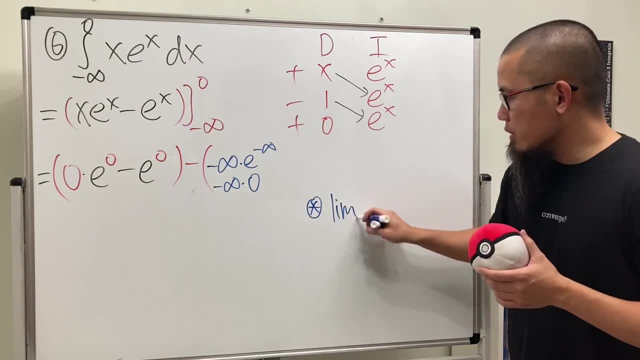 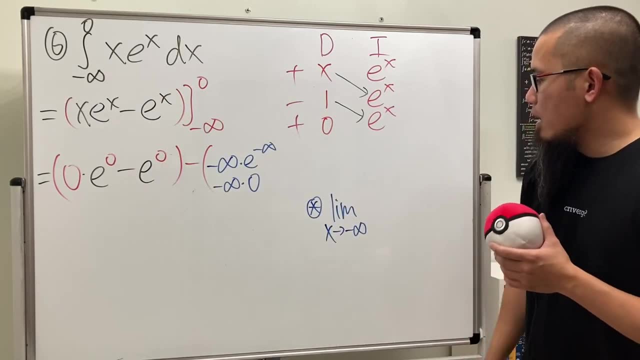 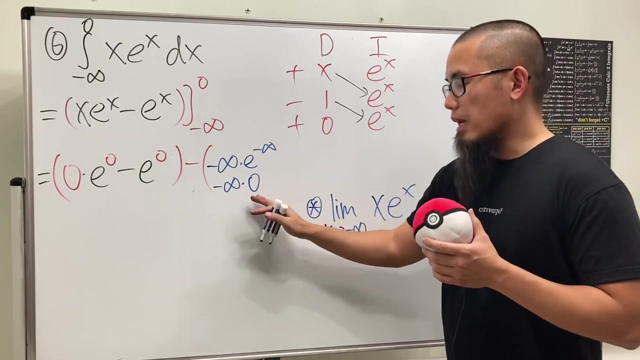 So let's do it right here: Put in the star, do the limit And let's just use x, As x goes to negative infinity and we have x times e to the x, And because this is a negative infinity times 0 situation, we cannot use Lapito's rule here. Maybe you can bring this. 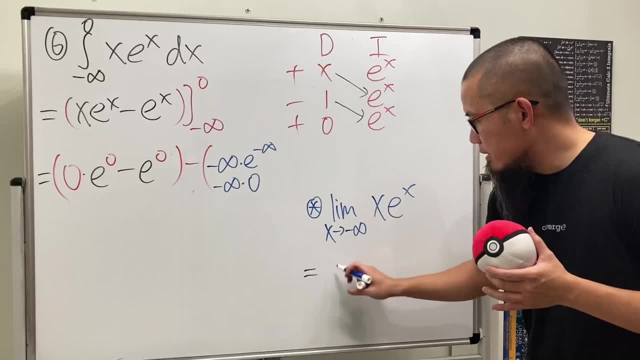 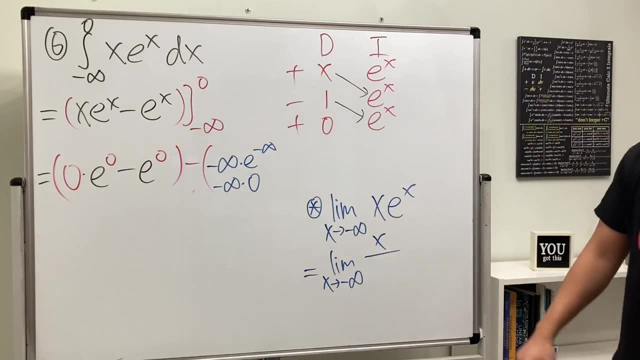 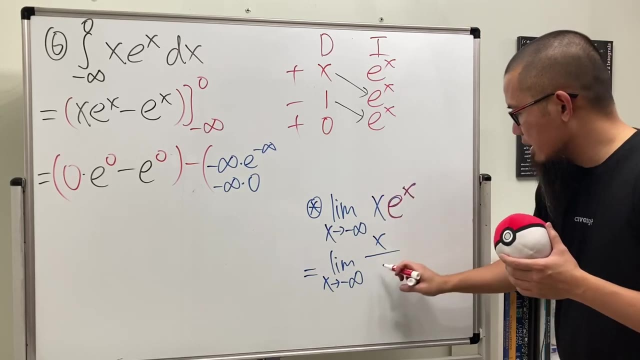 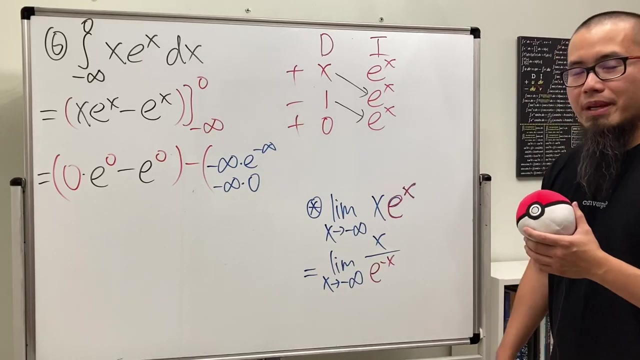 down, down. So you see this is the same as the limit as x approaching negative infinity. X on the top over. I'm going to look at the e to the x power as e to the negative x power on the bottom. That's cool, But you know what this is. It's going to be 0.. You can use Lapito's. 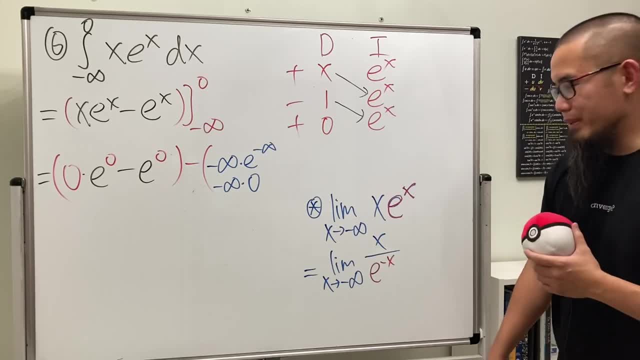 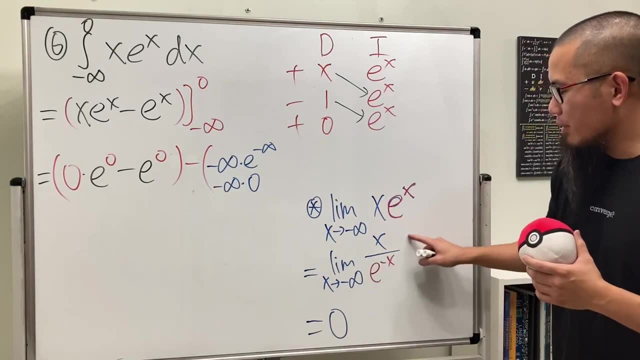 rule, But you know the better way, You know it, You like it too. This right here is just going to be 0. Why? Because now you see both, then is infinity and also on the bottom is infinity. But this is just the other version. 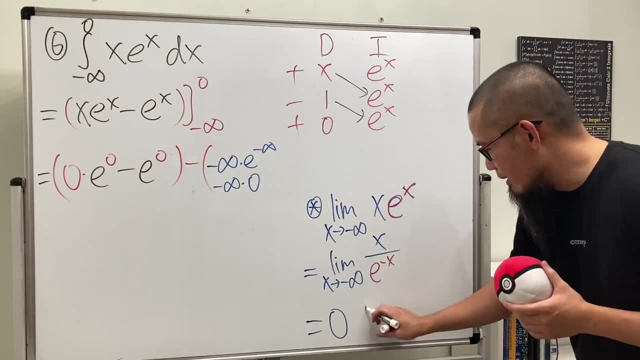 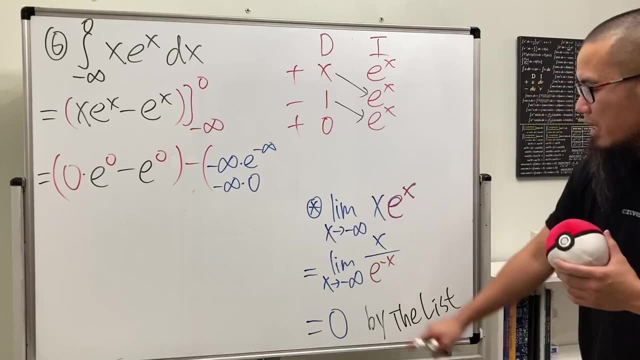 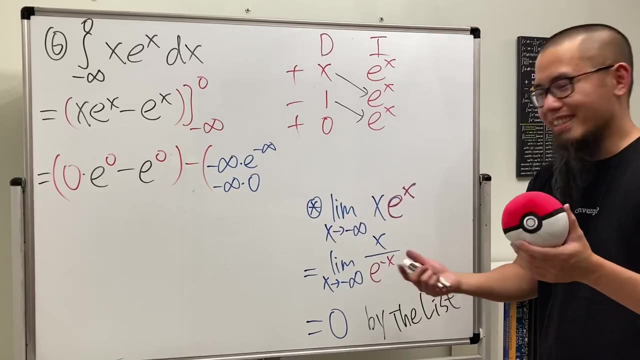 of the list. So I'll just say this right here is 0 by the list, Secret weapon. Again, if you look at this as negative infinity, you put it here. That's e to the infinity, which is just. it's really the same as the list. It's just you have a negative, but it's really. 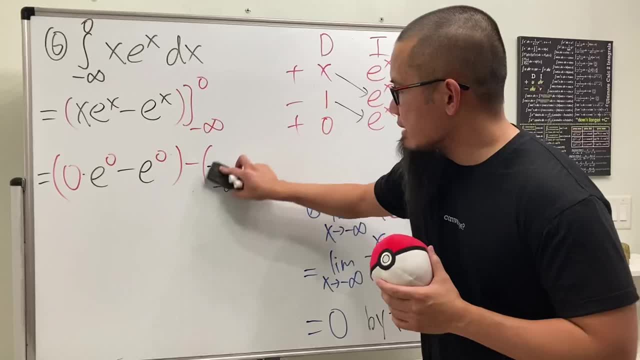 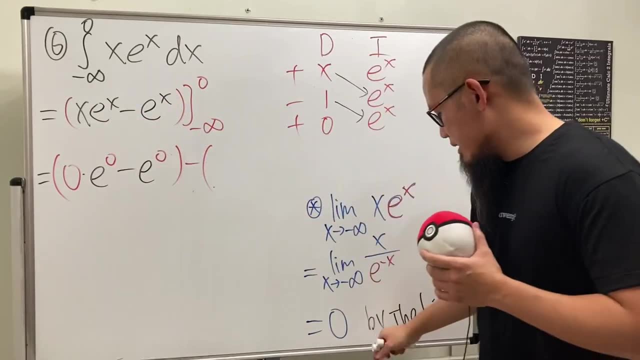 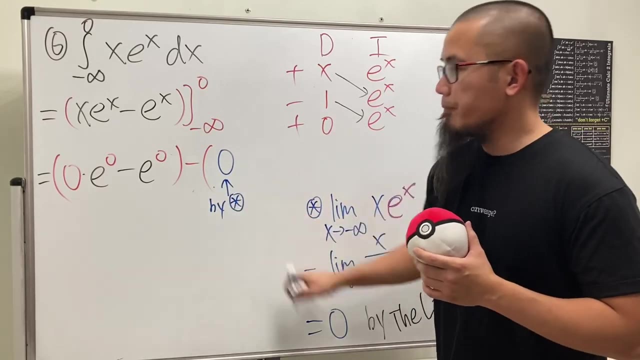 the same. So anyway, I'm just going to erase this right now. When you take the limit right- negative infinity of this term, we get 0. And then I'll just indicate that by the computation here, So by star, And then we put negative infinity there, We will have minus e and then negative. 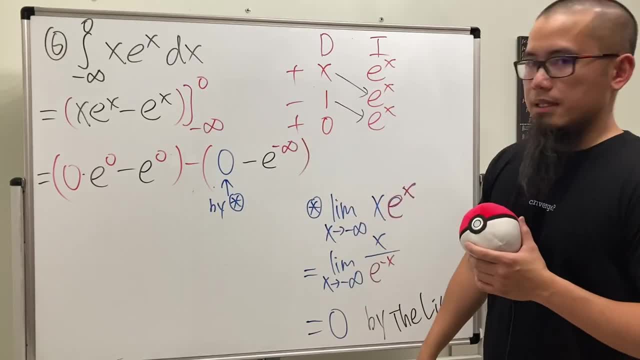 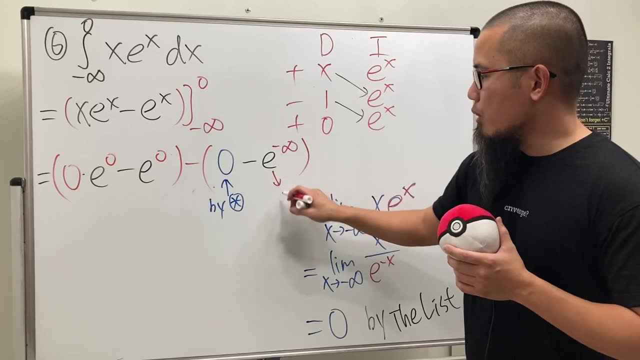 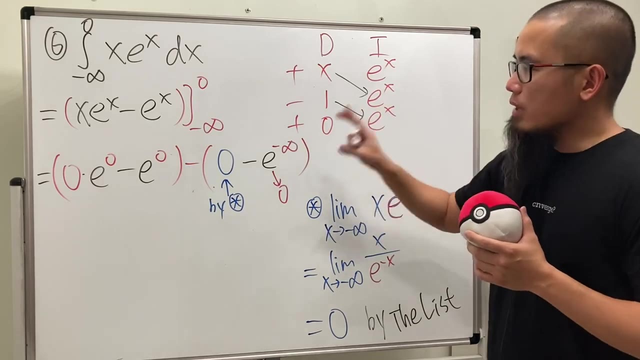 infinity right here. All right, Can we draw a conclusion here? Yes, e raised to a negative infinity, This right here will approach 0, because this is the same as 1 over e to the positive infinity, which goes to 0. So, luckily, the second part is just 0.. And then for the first part here. 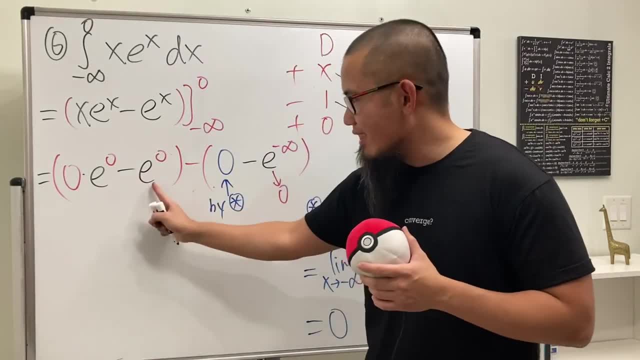 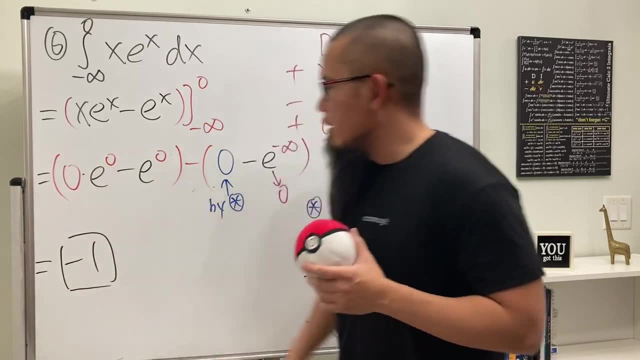 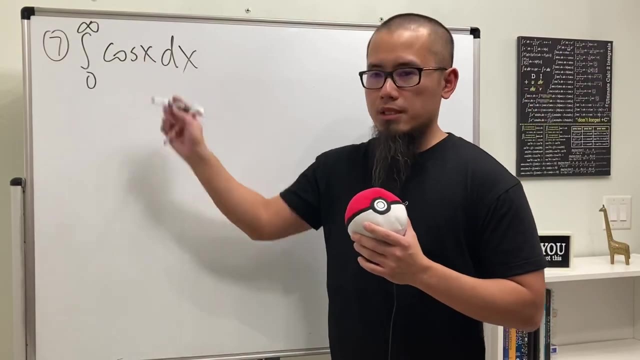 is 0, but we do have negative 1.. Therefore, ladies and gentlemen, the answer for that is negative 1.. A lot of work for just negative 1.. But that's it. Number 7, we have the integral from 0 to infinity of cosine xdx. 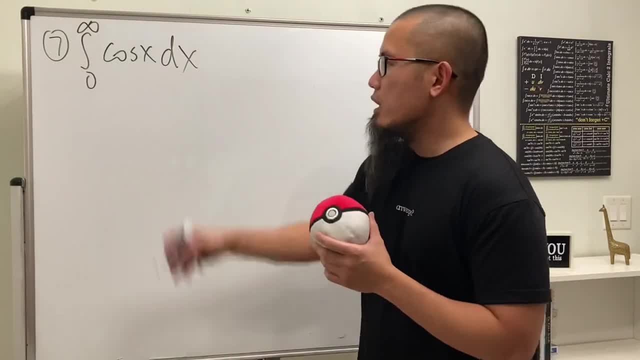 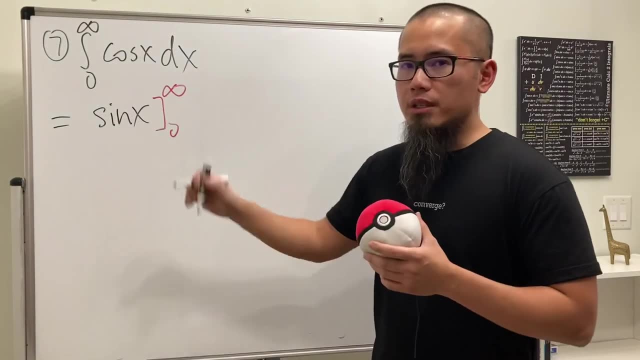 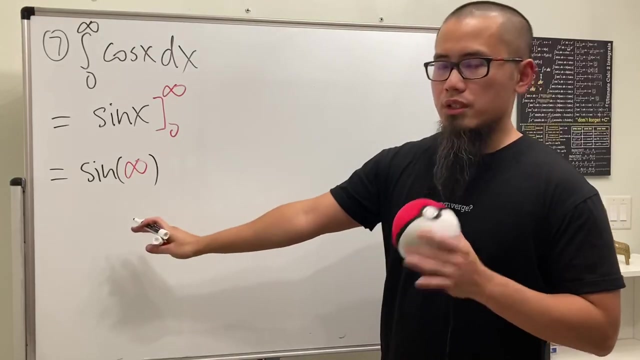 So of course we can just go ahead and do the integration. The integral of cosine x is just positive sine x. And then of course we are looking at 0 to infinity Drawing, infinity drawing 0. So we get sine of infinity like this. This is a really bad notation, I know. 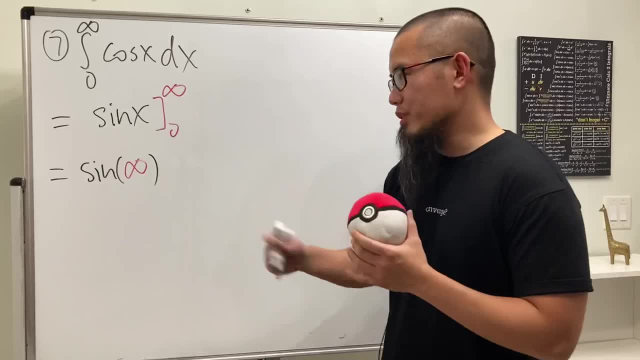 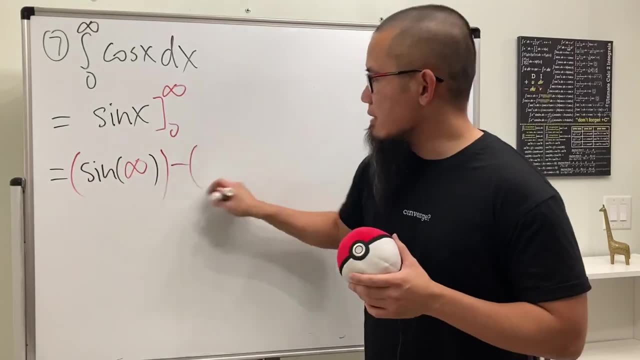 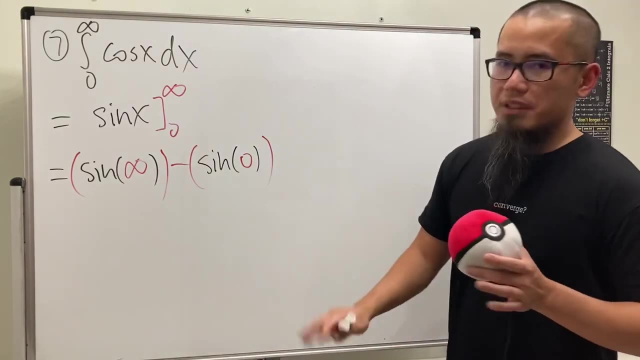 that. I said that so many times, but it's OK, It's just true. when you do all that stuff, If you remember that we are taking a limit, then this is OK. But anyway, first term minus the second, So we have sine of 0. Now this right here is 0. Easy, But what's this We do not have? 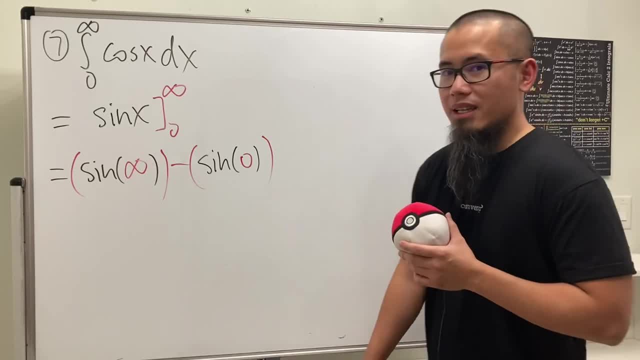 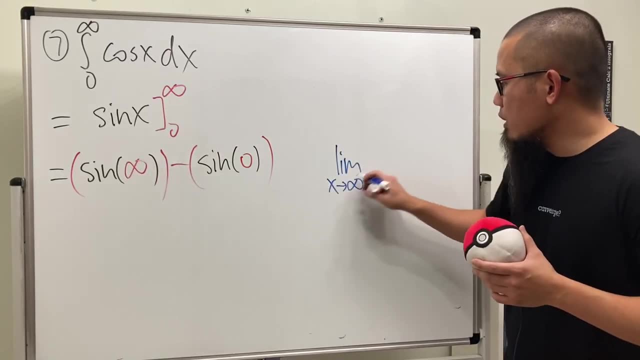 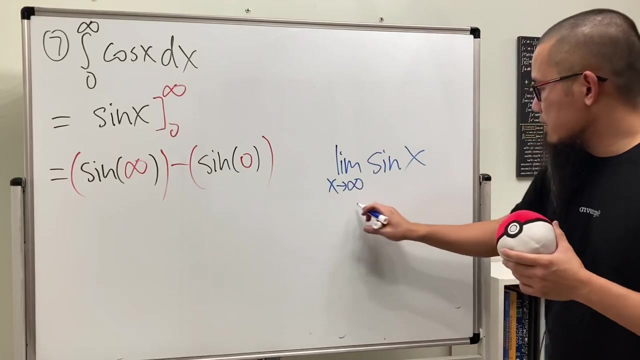 the limit for that. We do not have the limit for that. So when we put 0 in here, if you look at the limit as x approaching 0 of the sine function right- because we are doing that to here, not to this of the sine function- this right here does not exist. 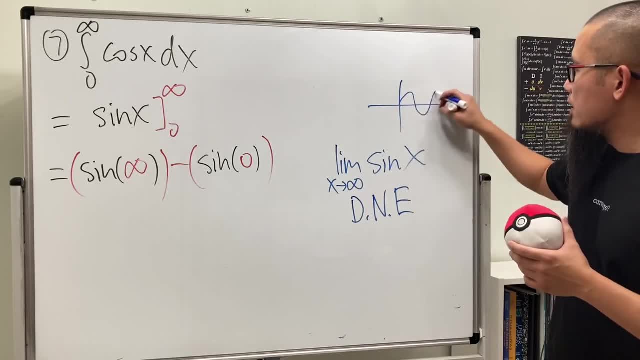 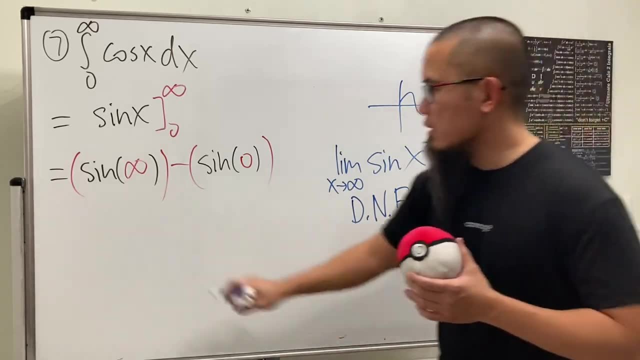 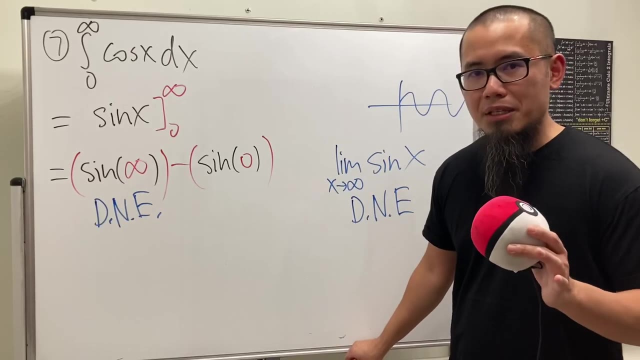 Right. Why? Because look at the graph. Sine x looks at this. As x goes to infinity, the y does not approach to a number. So this right here is d and箴. Well, d and箴 minus 0 is still d and箴. But don't do that. If this is d and箴, don't even look at these. 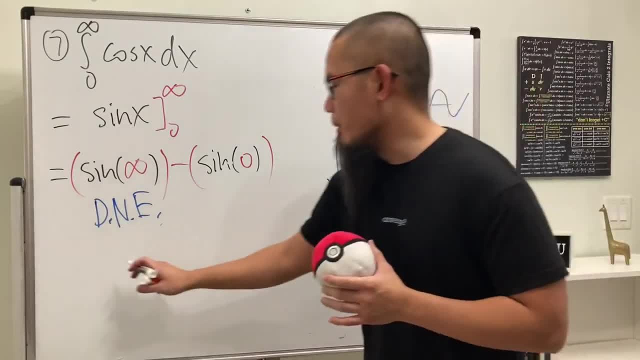 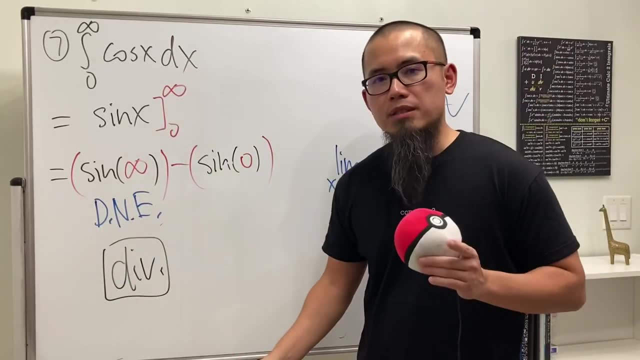 things, Just say: don't even say d and箴 for this, Don't worry about it. Come back here and just say this: integral diverges 0. chap 7.. 7 or 10 seconds, But please, please, please, please, don't ever say diverges to d and e. 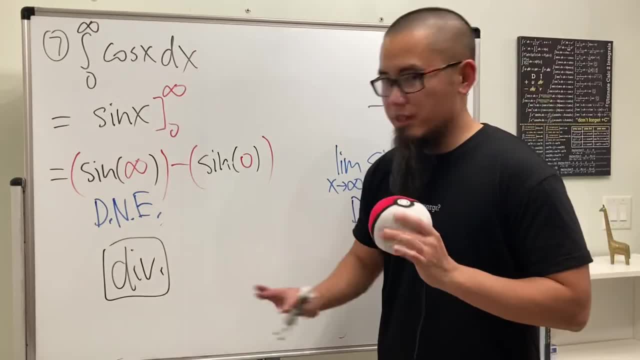 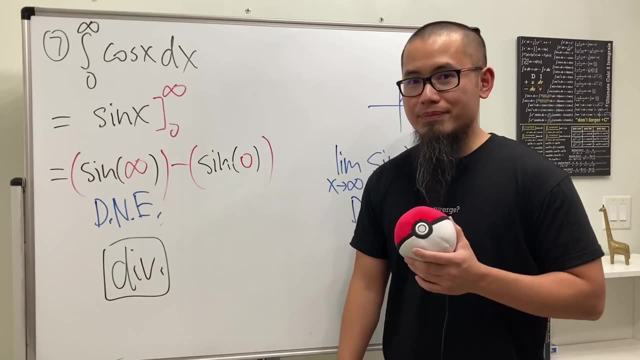 That does not make any sense. Just put on diverge, that's okay, right, That's okay. So this is another kind of divergent integral, right? You just don't get a finite value. Yeah, it doesn't mean infinity, though. 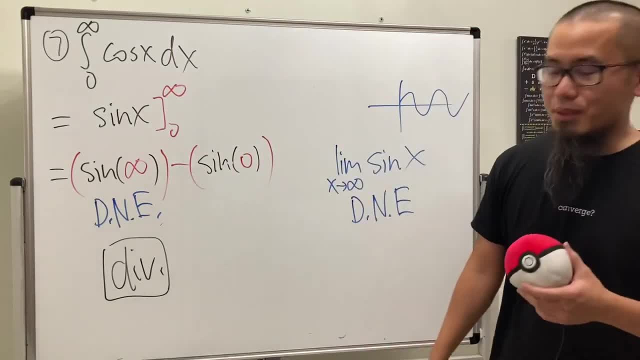 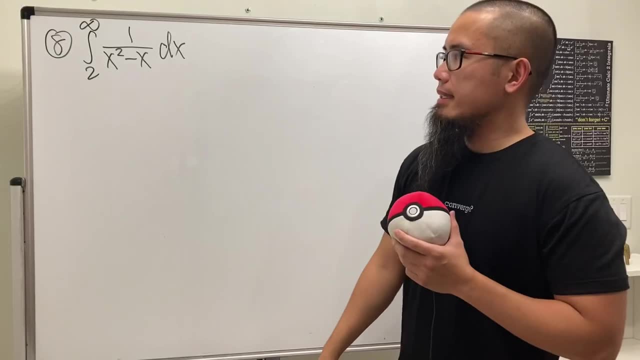 It's just that you don't have a finite value that this is approaching to. That's all. Number eight: we are going to integrate from two to infinity of one over x squared minus x. How do we integrate this? Well, look at the bottom. 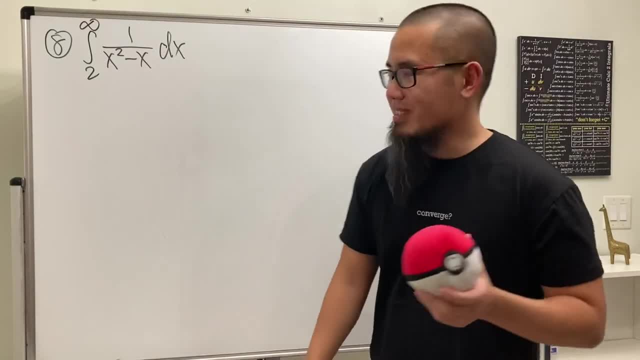 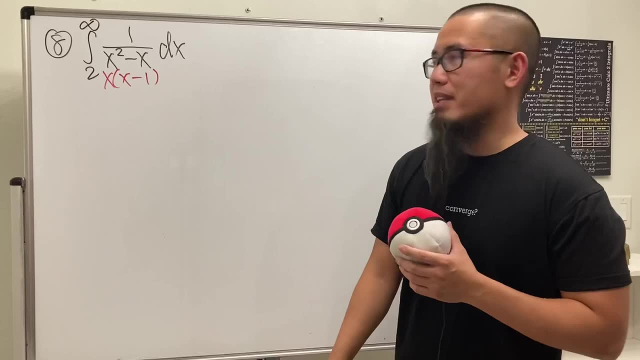 Can we factor it? Yes, So yeah, partial fraction. And it's not bad at all, because once we factor it we see we have distinct linear factors. So the partial fraction is not bad at all, right, Okay, so we look at the integral going from two to infinity. 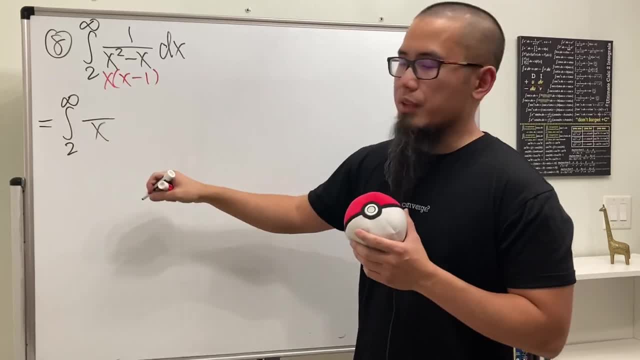 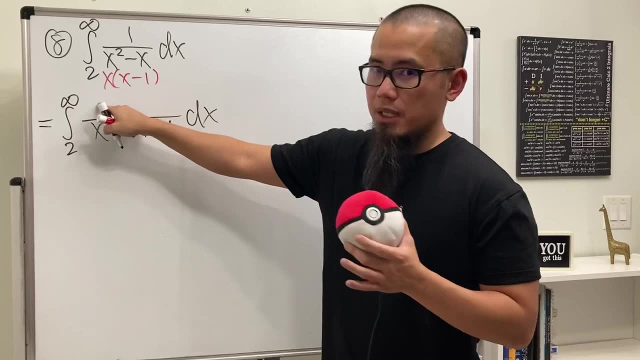 and the first fraction will have x for the denominator, and then for the second fraction, it will have x minus one for the denominator. To figure this out, which is going to be a constant, we look back to the original and cover the same denominator. 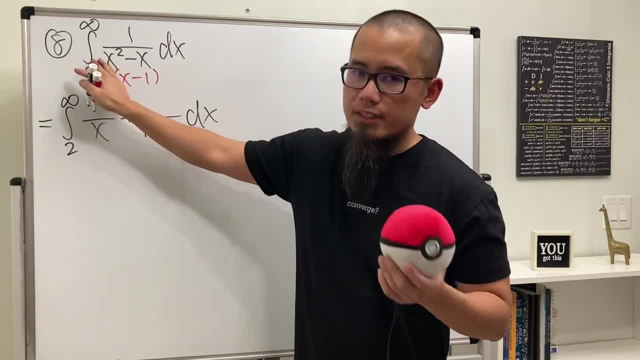 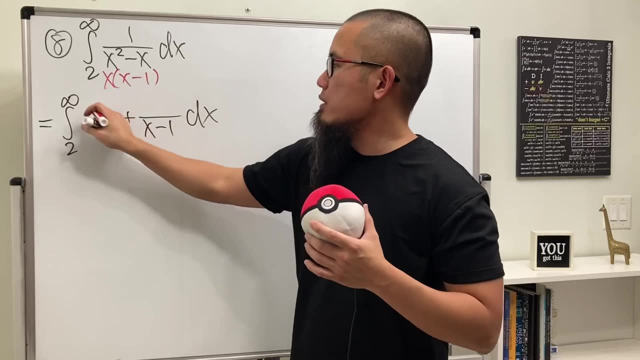 and you ask yourself: how can we make x equal zero? x has to be zero. And you put zero in this x, now One over zero, minus one, which is negative one. And then, to figure this out, we go back to the original. 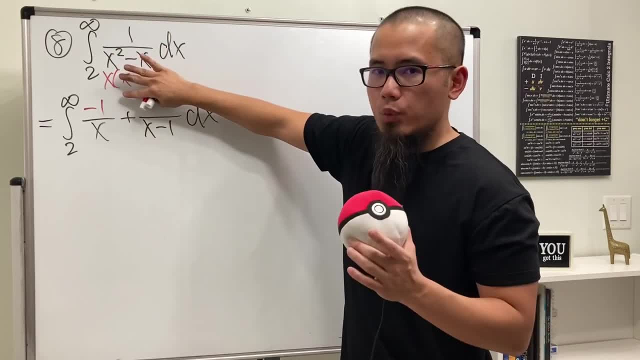 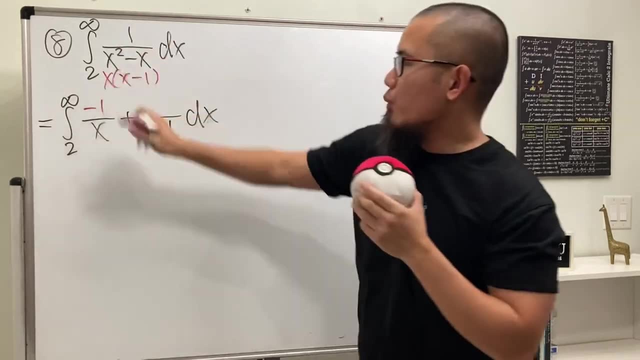 and then cover the same denominator and you ask yourself: how can we make x minus one equal zero? x has to be one. And you put a one in there. One over one is one Partial fractions. Now we can just integrate this: 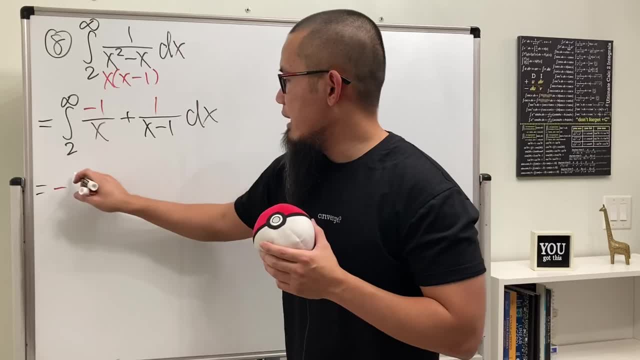 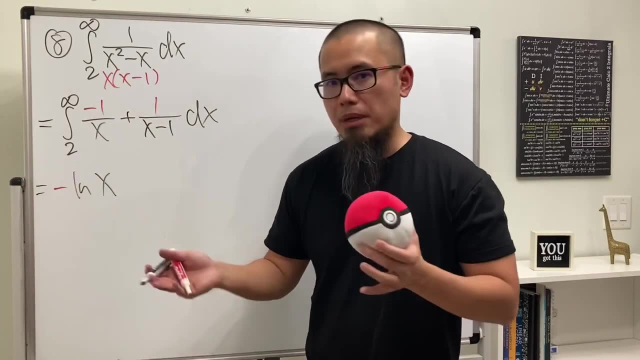 So we get this is negative and then ln x And we don't need the absolute value because we are going from two to infinity. so you know the x is going to be positive. Next we have to add one and then ln this right here. 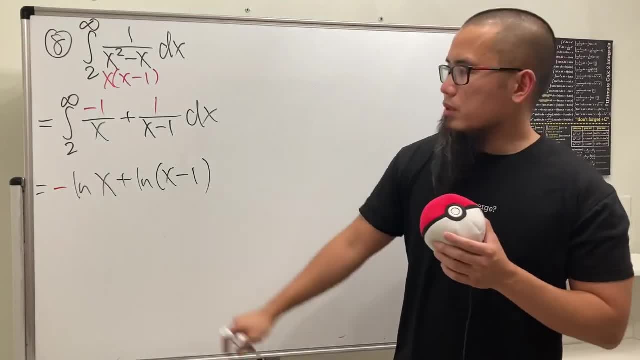 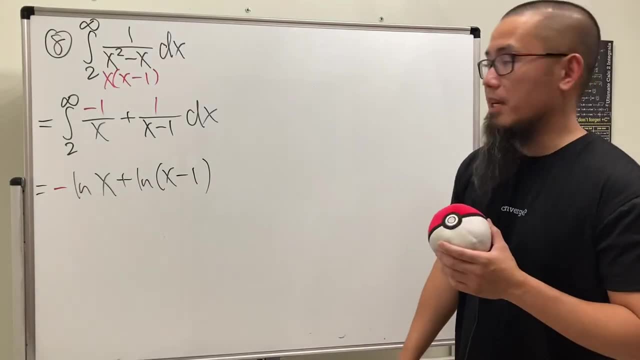 which is x minus one. And remember, you see, that the coefficient of x is just one, so that's why we don't have to divide it by any number. Okay, Technically, divided by two, We can divide it by one, but it doesn't matter. 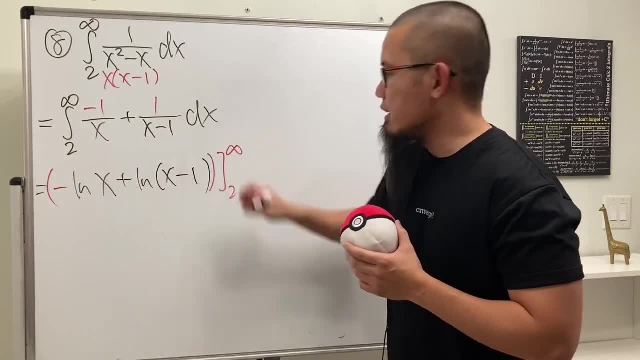 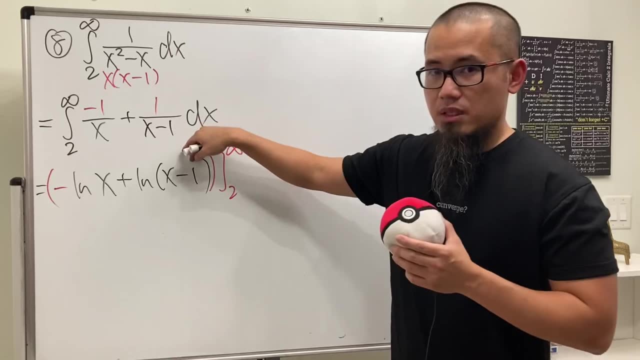 All right, and then we go from two to infinity, And perhaps, before we plug in infinity, we're going to combine the logarithms, Because if you don't, then if you have infinity, put it here, you get infinity and that's minus. 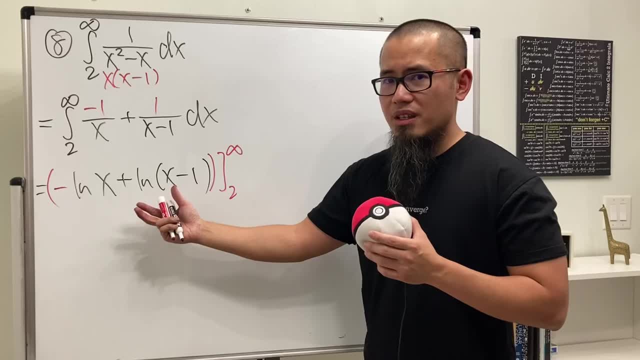 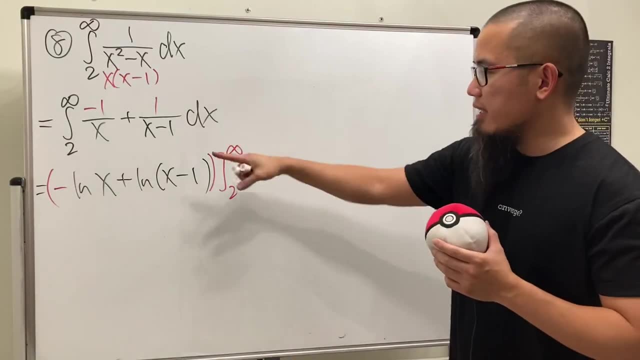 And then if you put infinity here, you know that's also infinity and you get indeterminate form. So we might as well combine the logarithms first before we talk about taking a limit. Okay, in that case, we see, put a natural log here. 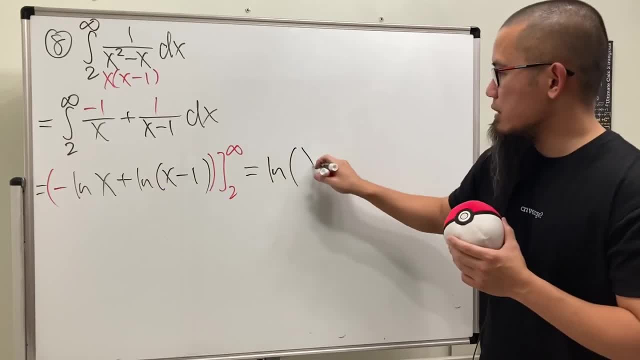 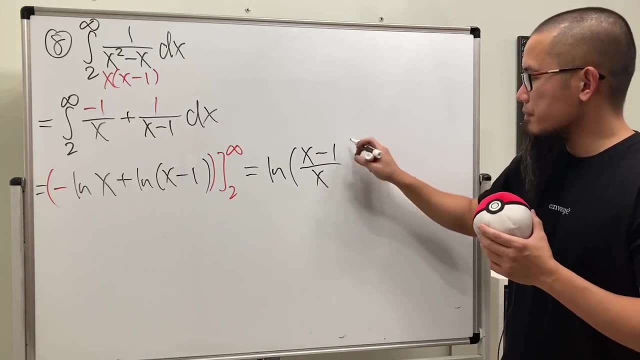 This will go on the top because it has passed the natural log right, So it's x minus one. And then because the minus ln x, so we will just have the over x right here, And then we go from two to infinity. 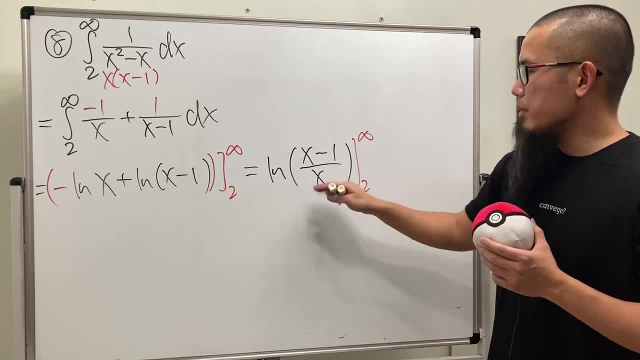 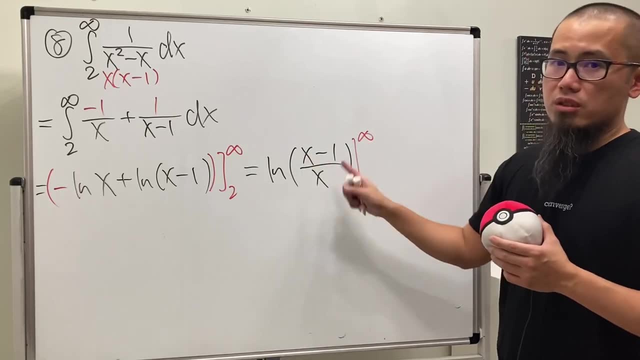 But this one's not bad at all. You don't even have to do l'Hopital, even though you are taking a limit when x goes to infinity, Because you see this right here can we split the fraction, Yeah, so perhaps let me just write this down one more time.